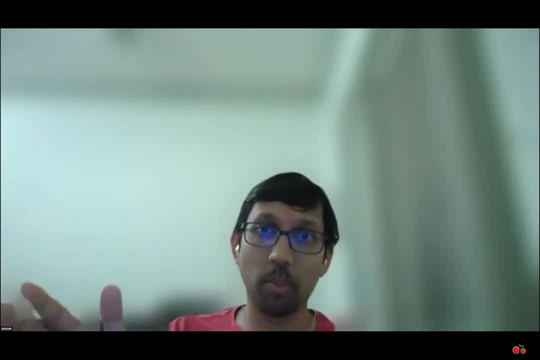 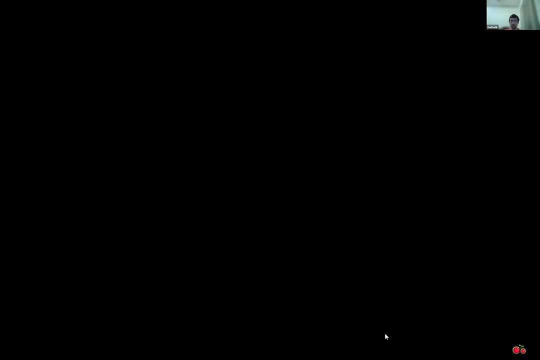 parameters. It doesn't have k, It has epsilon and minimum points. Those are the two parameters, right? So let me quickly share my screen And you guys should remember this figure that we spoke about last time. right, Two parameters: epsilon, which is the radius of the circle that you. 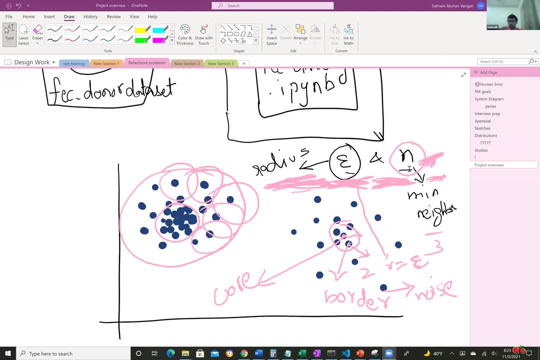 would like to draw and n or some kind of variable, which is the minimum number of neighbors that a point is assigned to. So that's what we're supposed to have, right? And you guys remember the three different types of points that the model detects: A core point, a border point and a noise point. 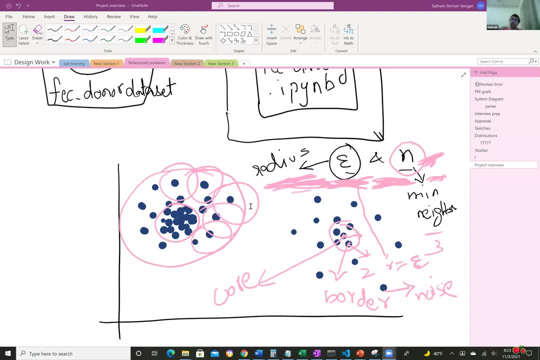 right. So, in every point of your data set, right the model, the dbScan model. and, by the way, dbScan's full expansion is density-based spatial clustering of applications with noise. Okay, You are not expected to know this, but it's good to know if somebody asks you in. 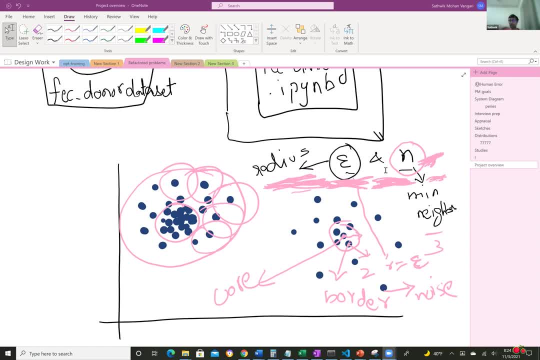 the interview. hey, can you tell me what dbScan stands for? You remember, in the last class I told you guys it's an acronym, right? It's density-based spatial clustering of applications with noise, right? So if you see, it's kind of intuitive, because this is one of the few. 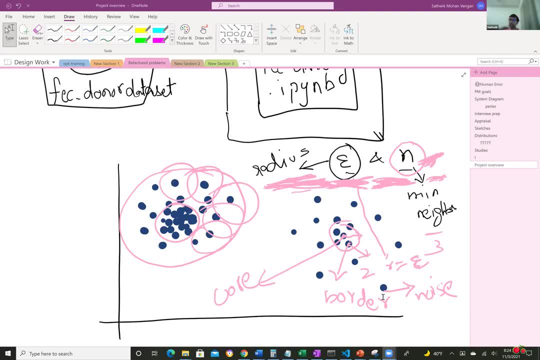 clustering models which detects noise and which doesn't cluster the noise, right? If you remember last class, we discussed this as well. that k means comes to a stop when the model has attached a label to every point in your data set, which means there is no. 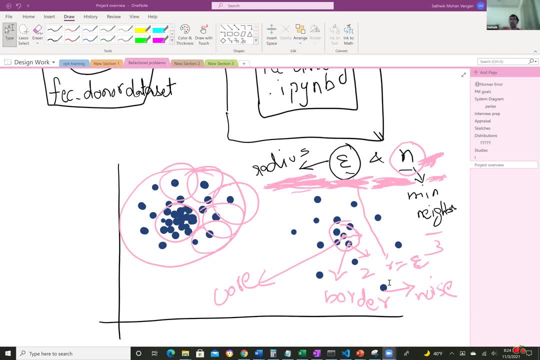 point that is left out. Every point needs to have one of the k labels. If it's three clusters, then you'll have three labels. You'll have one of the three labels, right? If it's four clusters, k equals to four. you will have four different labels, And every point. 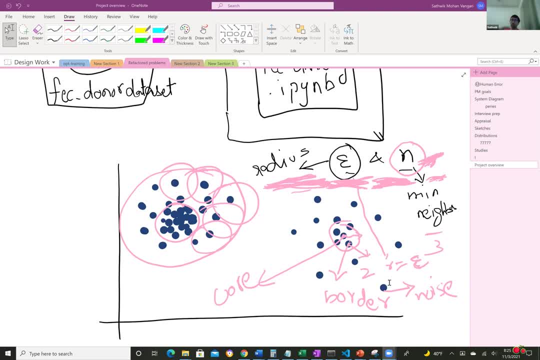 will have one of these four labels and every point will be labeled. And once every point is labeled by the model, that's when the algorithm stops right. So here, with respect to dbScan, it doesn't have the requirement or the need to cluster every point, So some points will. 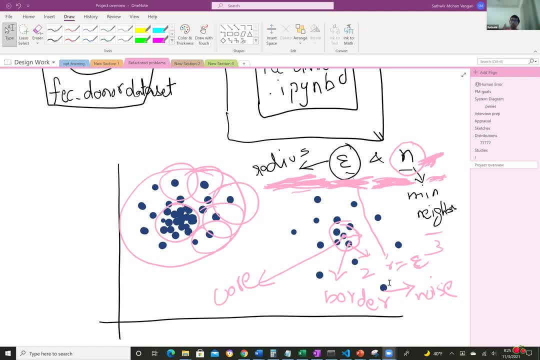 be left unlabeled. and those unlabeled points are what are kind of labeled unofficially as noise, right, So that doesn't, that don't belong to any specific group that can be seen in the data set. okay, Now, if you see here right, like, these are the two parameters as: 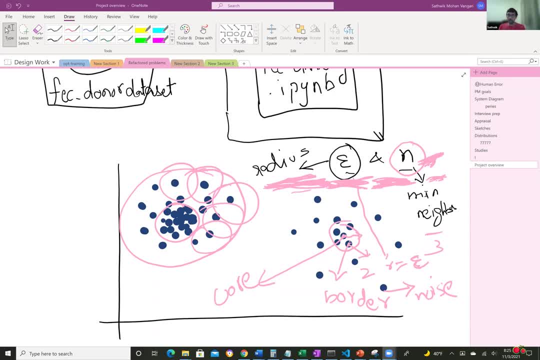 we discussed epsilon- the radius, and n- the minimum number of neighbors. there are three parameters that you need to have. So for every point, you draw a circle around that point, With the point as a center. you draw a circle around that point and that. 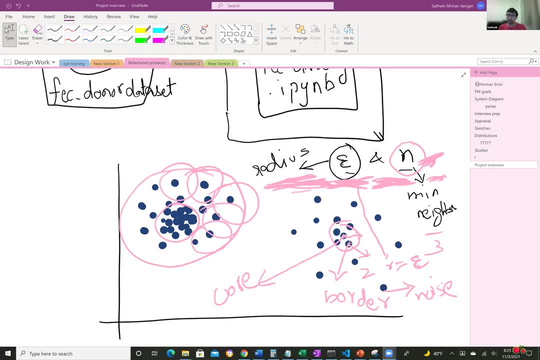 circle. the radius of that circle is epsilon. That's what you define to the model, right. So you assign a specific radius value, say one or two or three or whatever it is right. So if it's one, you see a circle with one unit radius. If it's two, you see a slightly 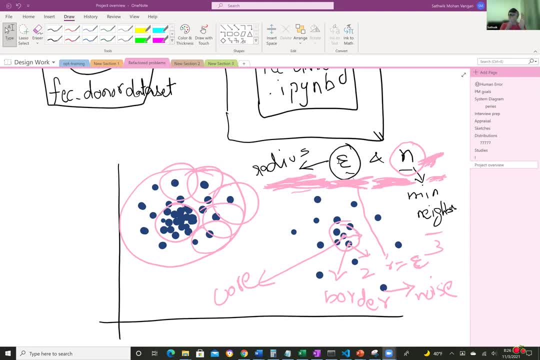 bigger circle Three, an even bigger circle Right. So, like that, the smaller or larger circle is drawn based on the value of radius that you prescribed right And based on that circle right. what you try to, what the model basically tries to understand is, once it draws the circle, how many points? other data points? 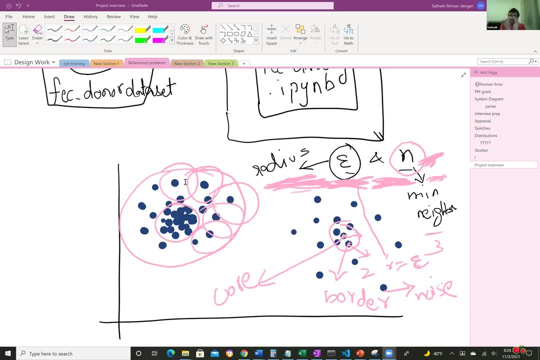 actually fall within the circle, fall inside the circle right. So if there are certain number of points, Same thing, number of or a number of points, let's say a number of points inside a circle. it tries to compare the number of points inside the circle for a specific point to the n or the minimum number. 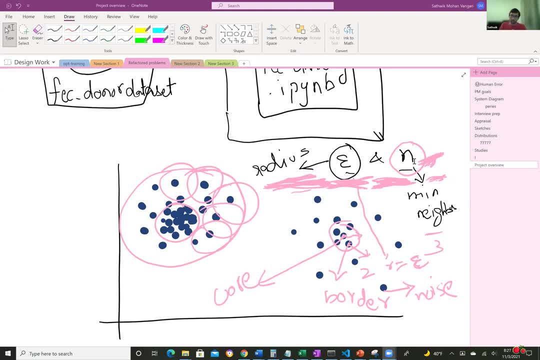 of neighbors that we have also defined as the other value. we will define. so if that a value, the number of neighbors of this specific, this specific point, right if it is equal to or greater than my minimum number of points, let's say, if i require minimum 10 neighbors, right for a specific. 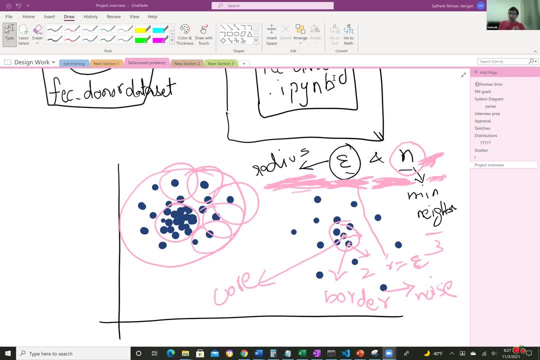 point. and if the point that i am looking at right now has only five neighbors within the circle, right, then i would say five is less than 10, which means that it is not satisfying this criteria. so it is not core to my cluster, right? or it is not a core point to the way i am defining or to 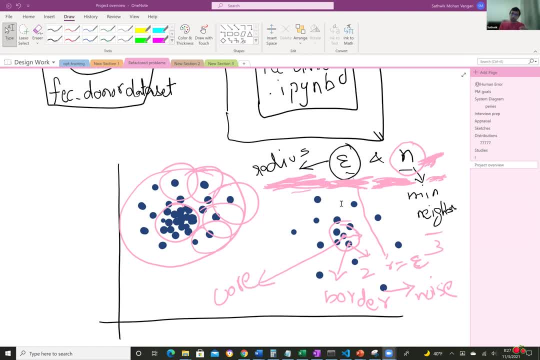 the way i want to define my cluster. okay, so that won't become the core point. it could become the border point if this point, which has five neighbors in itself, this point in itself is a neighbor to another point which has 10 neighbors around it in the epsilon radius circle, right in that circle. if this is one of 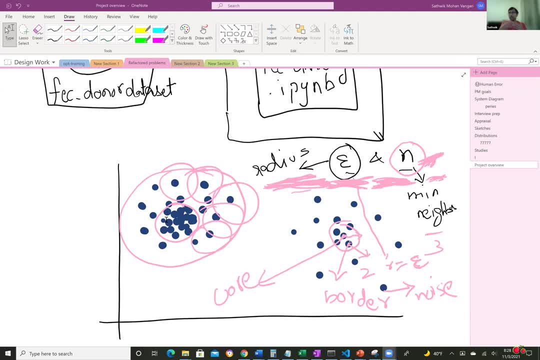 the neighbors, then it becomes a border point. and then there is a third condition where you draw the epsilon circle around the point, neither does it have the minimum number of neighbors required, nor is it a neighbor of a point which is a core point in the cluster, in which case that becomes 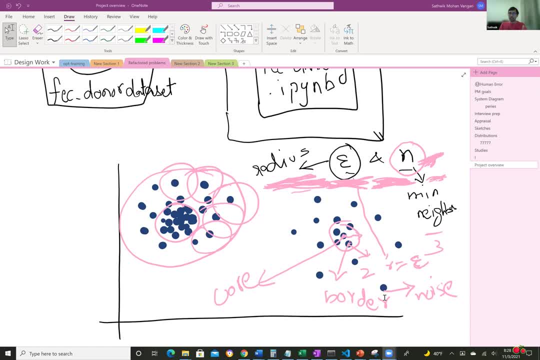 noise right. so these are the three ways: the points are classified by the uh, or rather identified by the clustering algorithm. and once these points are identified, what happens? the core points and border points together make the cluster right and they get labeled and the noise which is outside of. 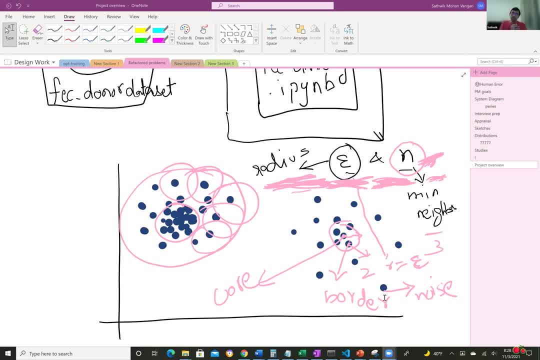 these points is basically unlabeled and left out, right. that is not supposed to be considered. that's just anomalies in the observations. that's what this is. so that's what db scan means and that's how it works, right, okay, all right, now i drew a circle over here, right, and let's say this: epsilon. 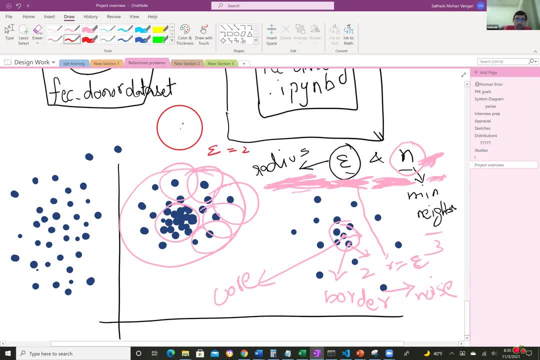 here is equals to two right, which means the radius of this circle is two. okay, let's assume that aspect. now what i will do is- i'm assuming that that's the point that i want to look at and this is my circle, okay, of radius epsilon. now my minimum points. minimum points, neighbor. i am defining it as six. okay, 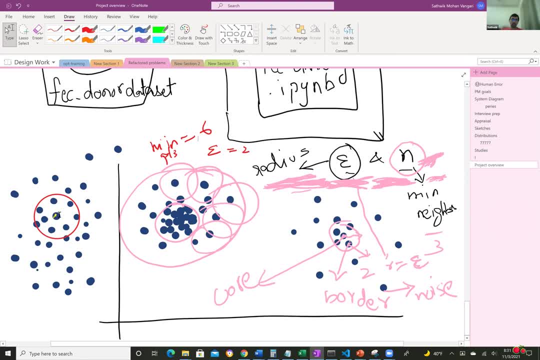 now, do we have a circle over here? now, do we have a circle over here? okay, i call this point as a core point or not? what type of a point is this? so this yellow point that i marked, is it a core point, is it a border point, or is it a noise? okay, it's a point, i think. 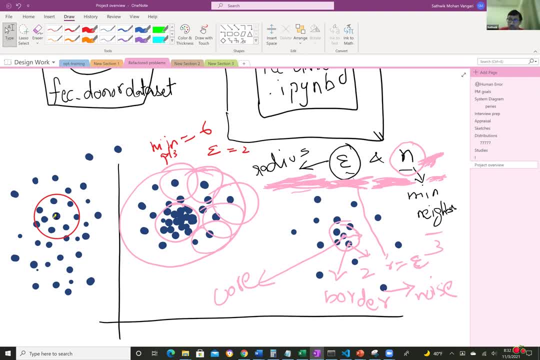 so who wants to answer? liz, you are answering. i said core point. why? because it's kind of in the middle of the epsilon circle. okay, no, that's not the reason. can anybody answer why it's a core point? so i'm right on the first one, right? 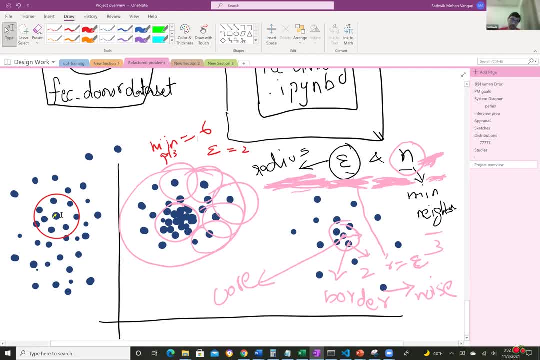 no, no, it yes, it is a core point, but why is it a core point? because it's inside the circle um, any of the points that are, i think, on the line of the border points. no, no, no, okay. so here's what i i will tell you guys. okay, i don't think you guys understood the concept. 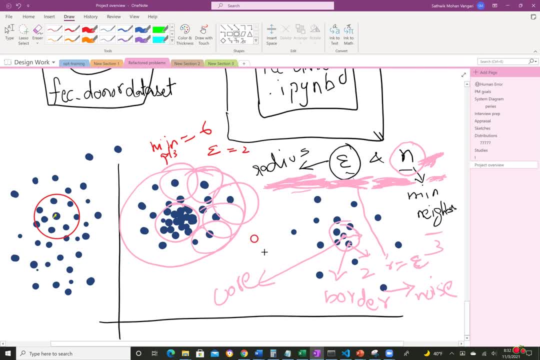 means four, like when you specified your parameters, like wasn't it one of the core points? and you say the epsilon was like three, two, so epsilon was two. yeah, epsilon is two, okay, two. so which is the radius of my circle? right, yeah, yeah, epsilon is two. what's the minimum point? it's the minimum number of neighbors, right? six, correct, okay, right. 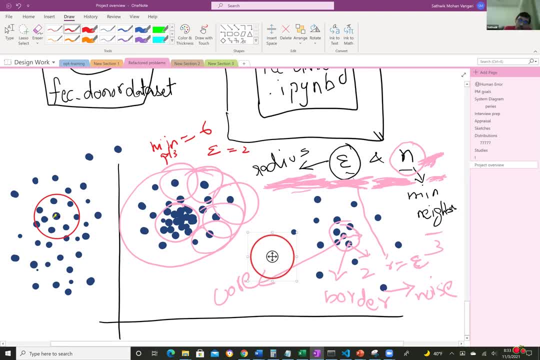 now, can you tell me if this is? this is my yellow point, right? that's the point that i'm looking at. how many neighbors does it have inside the circle six, eight, six neighbors, six and a half, count again seven plus. is it the first one or this new one? 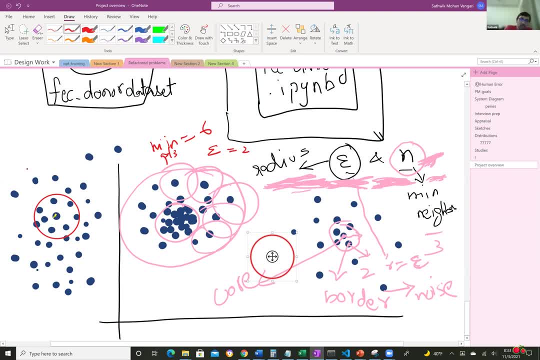 no, this, the new one, is just a circle that i drew. okay, this is my data. right, these are we counting the, the, the yellow thing as a neighbor? no right, no, no, that's the point i'm talking about. so what are the other points inside the circle? and that circle will be, uh, the minimum, because 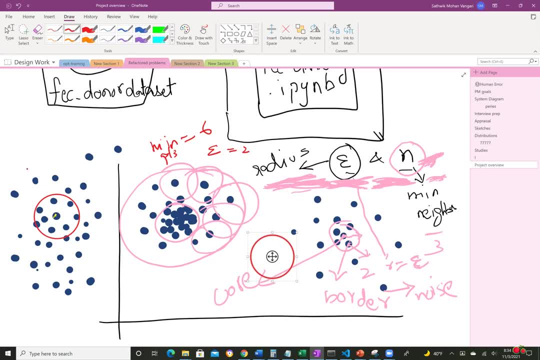 inside the circle. it has a minimum. see, the circle's radius itself is two, which is here, okay. okay, the circle's radius is two. forget about the size of the circle. minimum points is six. okay, how many points are there? jude, you were saying seven, yes, yeah. so can you guys count seven points inside the circle? everyone eight, yeah, seven. 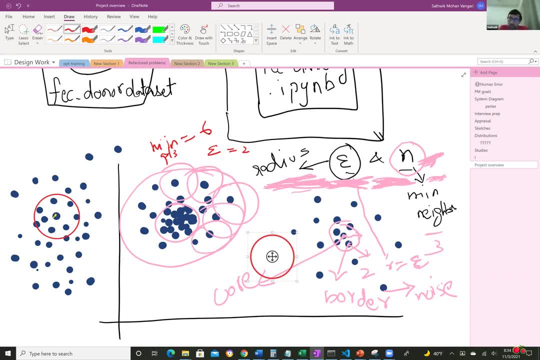 seven and a half, like yeah it's, it's on the border. maybe you can consider it right, maybe eight right, because it's a big point, uh, because it's a big thing that i drew it kind of looks seven or eight right. roughly now is seven or eight equal or greater. 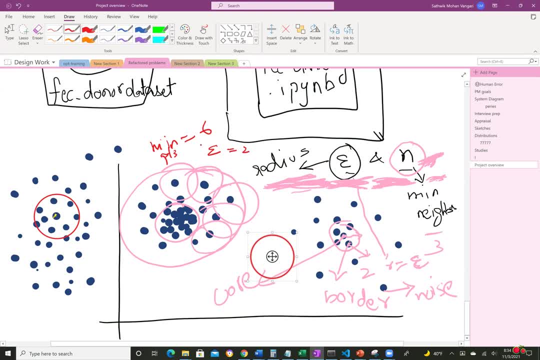 than six. it is right, yeah, now. does that satisfy my number of neighbors condition? yeah, because you said minimum six, exactly. so what does that become? that becomes the core point right now. yeah, so it is. that's why it is a core point. you get the idea now? yeah, so you. 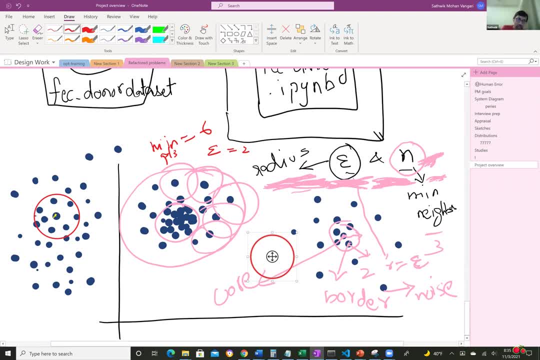 you, you, you label a specific point, a score point. if you draw the circle right, like you are drawing, we are putting the circle around that point right and we are saying that, okay, how many, um you know, neighbors does it have inside this sized circle? a two radius, two unit sized circle. 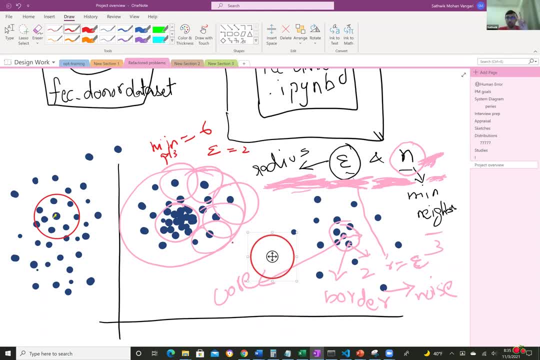 let's assume that the size of the circle is two, right, the radius is two. but let's assume the size circle is two, right. if the size of the circle is two, with a two sized circle, how many neighbors does it have? does it have six or more? it does have more than six and that's why it's a core point. now let me so this circle. 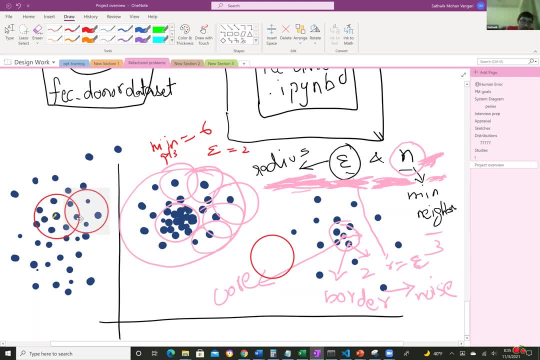 is kind of very similar in size, right? okay, so again, this is a two-point circle, right? look now let me draw, put it here, okay, how many points do you see inside the circle? you mean inside the intersection, or which circle are you? no, no, no, inside the circle that i'm moving. 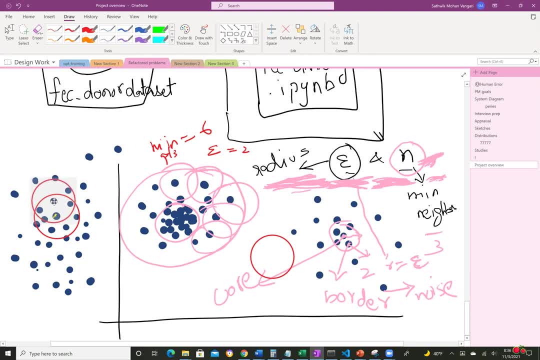 right now, four, five, yeah, yeah, four or five. nonetheless, four or five, right, yeah, yeah. so what's the minimum points? the minimum is six. it doesn't mean six exactly. so when it doesn't meet the minimum, is it a core point or a border point? but it's not a core point because it doesn't mean. 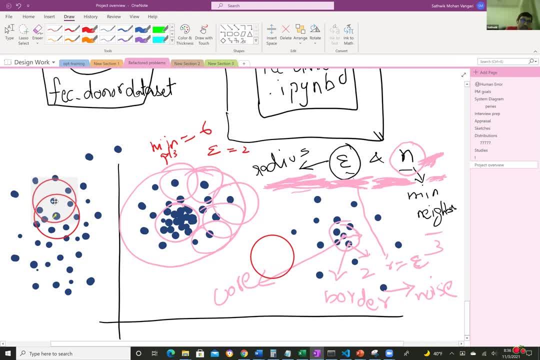 the minimum, correct. so it's a border point right, the next best thing, the border point right. so, uh, what is it? what are we uh parameter for a border point? parameters for a border point is: it doesn't meet the minimum neighbor's criteria, right, but at the same time it is. 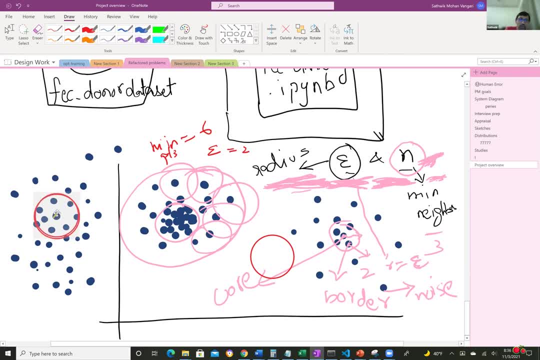 in the circle of another core point, right? so this point here it's in the circle of, and it is a neighbor of, another core point. yeah, i think i think i understand now so, but it's a core point if the number of points within that circle satisfies the minimum number. 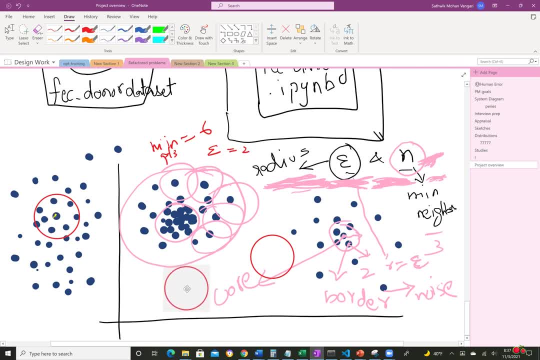 so if you have a minimum of six, then okay. does it mean all the points with except without? all the points inside are core points? no, no, just not all the points, just that point. okay, right, this the most central point, that's the core point. yes, okay, see, and and why does? 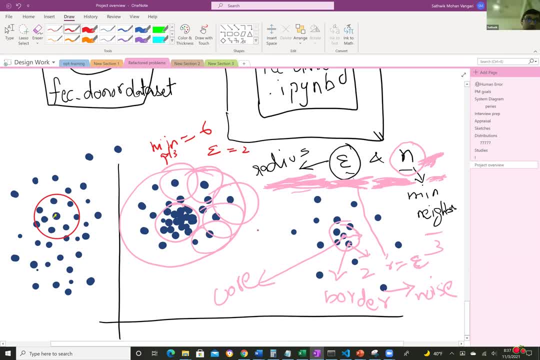 the. let me do this. why does the center even matter? okay, because you're drawing, you're trying to label, or you're trying to identify or classify each point, right? that's what the model is trying to do. so it first. first, we are trying to draw for this point. next, we'll try to draw for this point. right, then we'll try to drop from this. 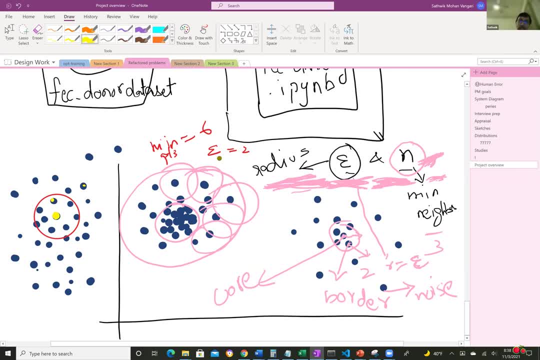 point like that. for every point we will draw a circle with the radius of two. we will draw circle, a two-sized circle, right, and then what we do is, once we keep drawing these circles, we'll check how many neighbors it has, right, so this one has like about seven neighbors. so it's a core point. 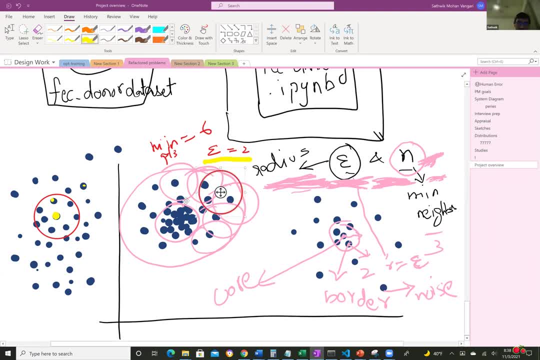 right, the next one, right, the next one, which is this point, right? it has like four or five points, right? so that point is not satisfying the minimum number of neighbors condition, which means it's not a core point. i'm talking about this point here, right? so this becomes a border point. 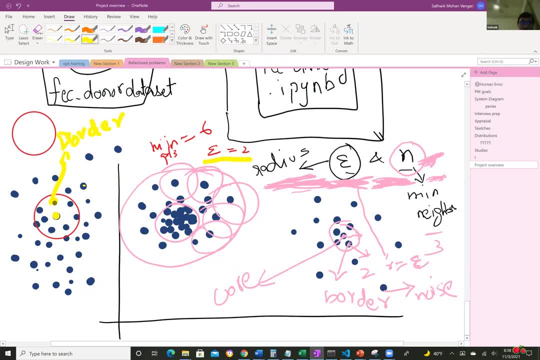 okay, because it's not satisfying the minimum number of neighbors condition, but it is a neighbor or it is present in the circle of another core point. now, this point i marked as core right initially make sense guys. now, uh, sorry, sorry, sorry, sorry, can i ask you a question? yes, okay. so based on that principle of uh, the number of point, 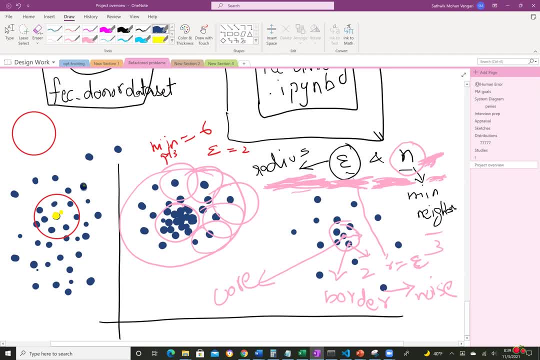 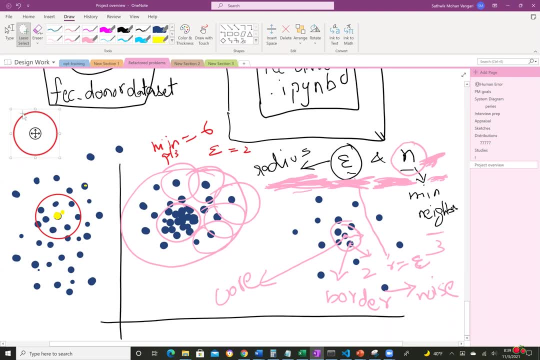 meeting the minimum of six. now, within that, within that same circle, let's say that we remove three points. okay, three points, three, three point. we remove three point out of that circle and we have five, including. yes, go ahead and do that, yeah, yes, okay, uh, one more, okay, so we have five. 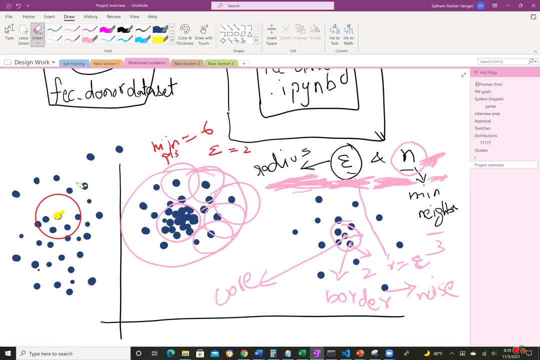 solid point and then the circle is crossing one circle. how is this a- uh, a core point? okay, this is not. now, it is not a core point. why not? because how many neighbors does it have inside this particular circle? you have five and it's crossing. it's crossing one, correct, right, but what's the minimum criteria that i'm looking at number six. 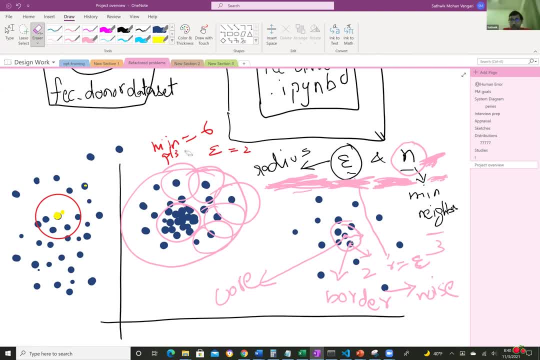 right, six, yes, six points. so it doesn't have six points in its neighborhood. so this can't be a core point in a core point any longer. right now, if i just oops, so quick, quick statement, so, uh, in that, in that principle, if, if, uh, the circle is crossing a point. 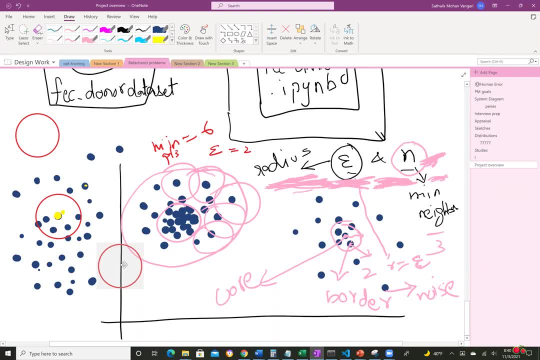 we should totally disregard, right? so the thing is, if it is on the point, you can consider it to be in the neighborhood. okay, that should be fine. but again, how many points are on the circle now in this case, even if you consider the, uh, the point? see, here i drew the points to be pretty large. 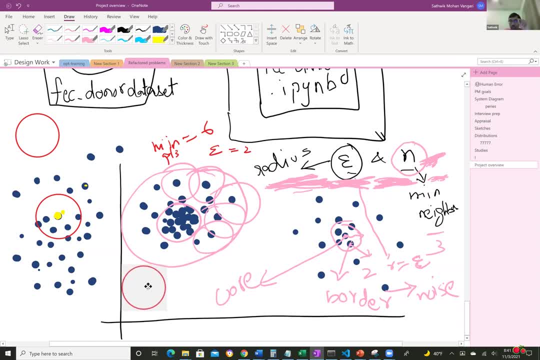 right. in reality, a point is just a speck right just so that we are able to see. i drew the points like that right so we are able to see that. we are able to see that we are able to see that we are right. but i ideally like: how do the how would the points look? like um points would typically look. 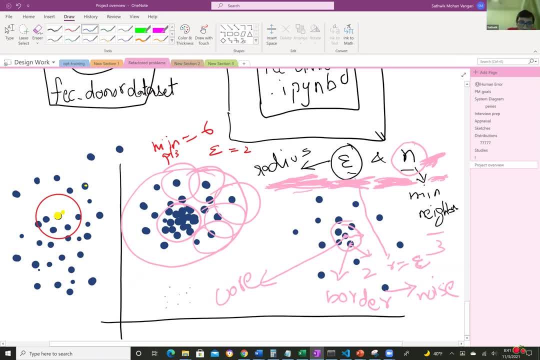 like this: okay, now do you think that the circle might probably possibly cut through them? no right, it might happen. it's not impossible. it might happen, in which case you can assume that the points are in the neighborhood and you can. you can count them in as neighbors. right, but it's up to. 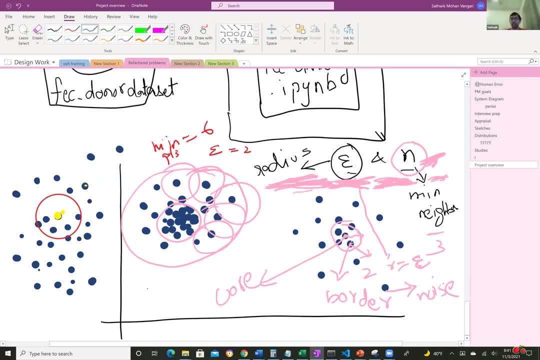 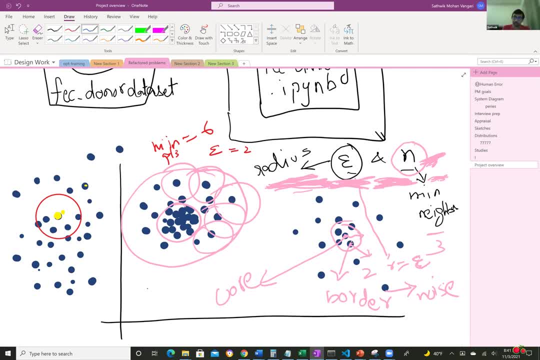 circle as well. it assumes that they are in the neighborhood, right, but in this case? so assume that in this case, even if it's cutting that point over there. so let's assume one, two, three, four, five and let's say six, right if it is. if we assume that this point is also counted, and if it is, 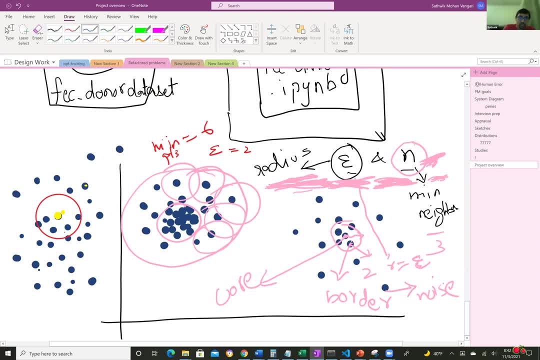 you know, uh, if it's the sixth point, it's meeting our minimum minimum correct criteria. in that case, it is a core point is. did that clear your question? yes, it makes sense. i just wanted to understand the uh, the exception. yep, so that's the yeah, that's for the first point. right now it's not. 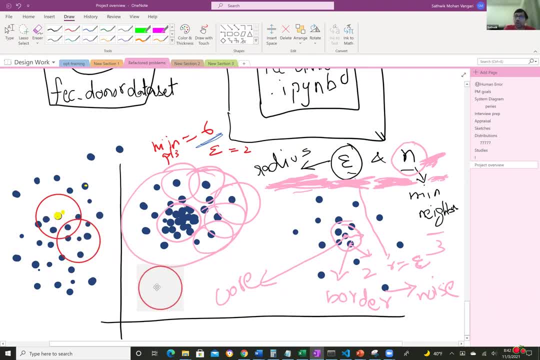 that the circles will overlap each other. you have only one circle at a point at a time, right? so like, if you guys remember the k means thing, right, we had iterations right in one iteration. in each iteration we pick a new point, we assign it to some cluster and then we move on. right is the same concept here as well, in the 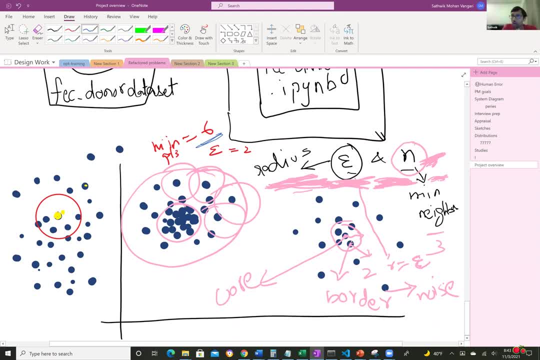 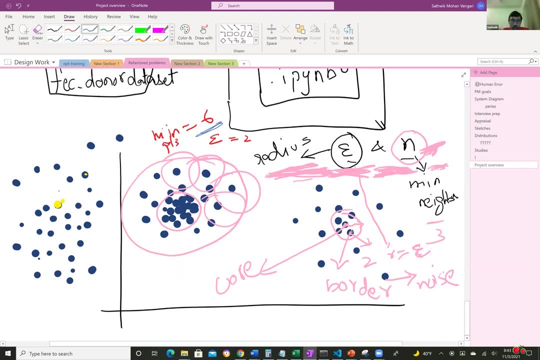 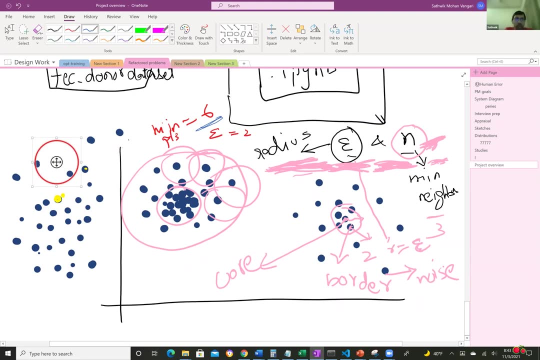 first iteration: i mark this point as either border, core or noise, right. and then what i do is i get rid of that circle. now i know that that's a core point or border point, right. then i move that circle to another point. i put it around this point. okay now. so if that's my point, right, you? 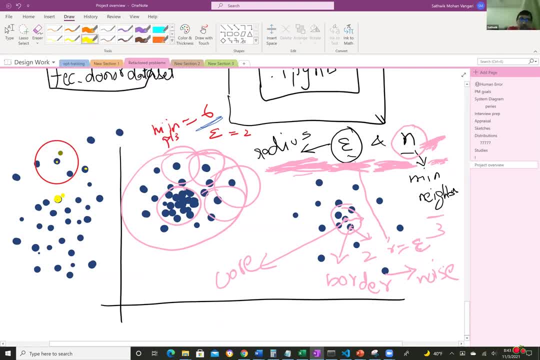 understand now which point i'm referring to, right, the point at the center, right? so, if that's my point, how many neighbors does it have, guys? how many neighbors does it have? where's the point? this, this yellow here? okay, he only has one with the red circle around it. one neighbor, maybe two neighbors, right? yeah, maybe two neighbors, maybe. 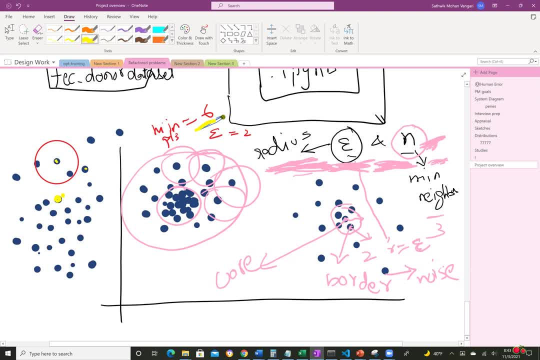 two neighbors right now? two doesn't satisfy my condition here, right, no? and is this a neighbor to another core point or even a border point? no, right, no. but it depends. assuming we have another circle around here, it could be, yes, but if you see, you know it's, it's a neighbor, its neighbors are this point. 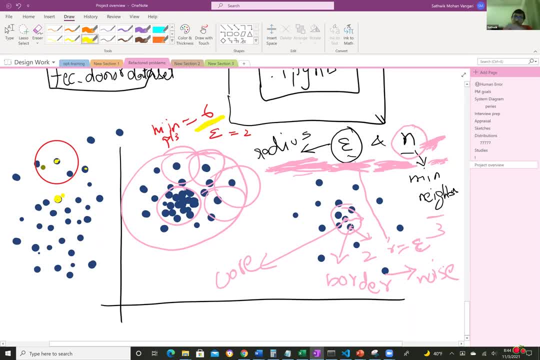 and this point, and if you put circles around them as well, right, you don't. so this point is also not a border point. this is also not a border point. so and this point is also not a neighbor of another border point or core point. it's pretty far from all the main stuff, right? that makes this a noise. 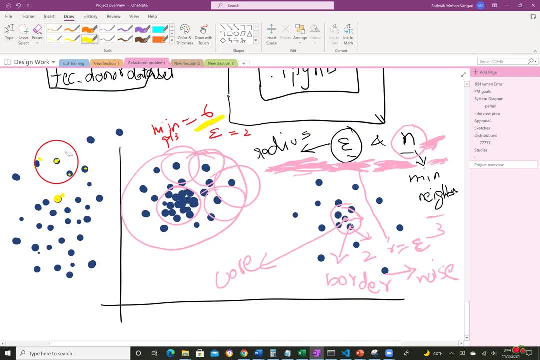 okay, okay, right. so, um, let me check. give you another example, Let me pick this particular point. Okay, now, let's assume it has five, five points, right Five, neighbors, Right Five, which means it is not satisfying our condition. But but let's pick this particular point Right Now, this point here, right? 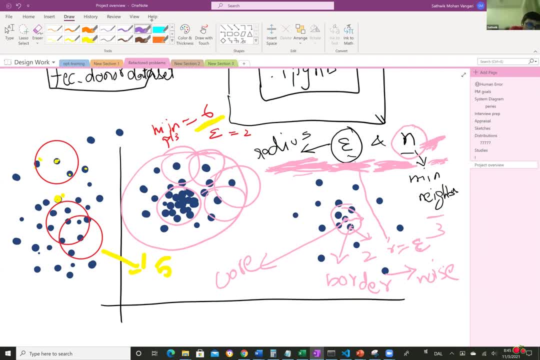 Okay, let me use a different color. This purple point here, right? Is that a core point or a border point? Okay, guys, this purple point here, is that a core or border? It's a border. Why do you say it's border? 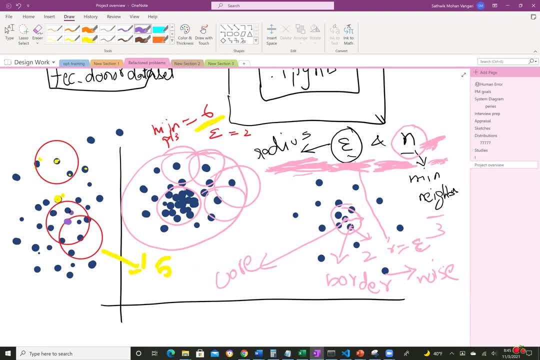 Because it's not a core. It doesn't have. How do you say it's a border point? It's a core point because you have six. Exactly right. It's a core point because with the circle around it, so don't look at other. 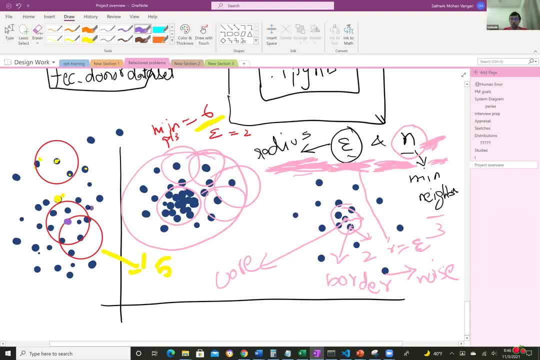 circles. okay, Border point doesn't mean that a point which is on the edge of the circle. No, That's not the idea here. right? These circles are drawn just to show you the neighborhood, right? Just to give you an idea of neighborhood In reality. do you think that the model is? 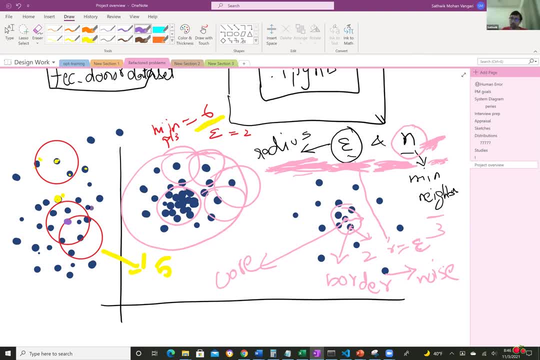 actually going to draw a circle and check whether the point is falling on the border or not? No, right? No, It's just going to look. it's going to look in the vicinity right. The circle is just to tell it how far it should look in each direction. Make sense, guys. no. 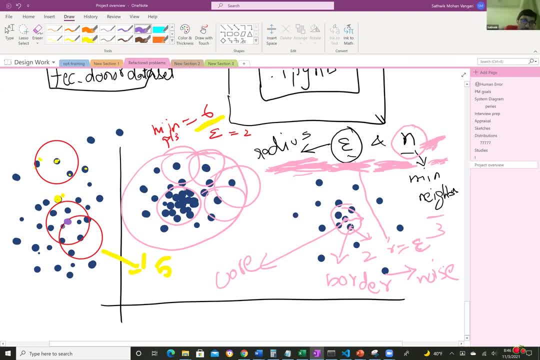 Yeah, So with respect to this particular purple point and the circle around it, it has six points or more around its neighborhood, right, And and one and so it is a core point, And one of the points is this: Let me draw the brown point, This point right, This brown. 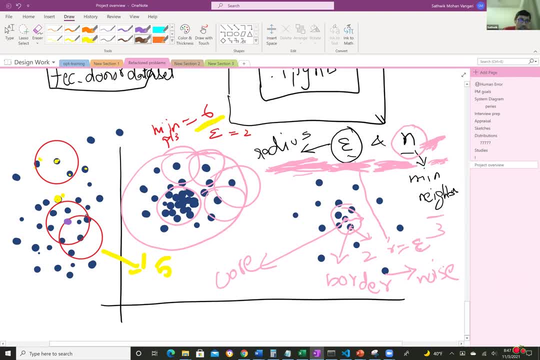 point. Okay, Oh, brown is not visible, Let me draw orange. Okay, It's that orange point. Right, One of the neighbors of this point is the orange point right Now, because so this orange point here has only five neighbors in its circle, which means it is not satisfying. 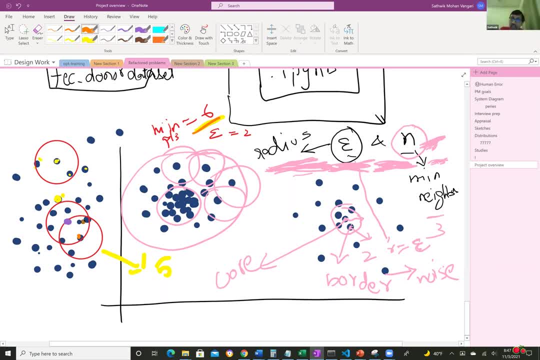 the minimum neighbors condition. So it's not a core point, but it is a neighbor of a core point, which is the purple point, right? So what does that make the orange point? It makes it a border point, correct? No, Now, now do you understand? 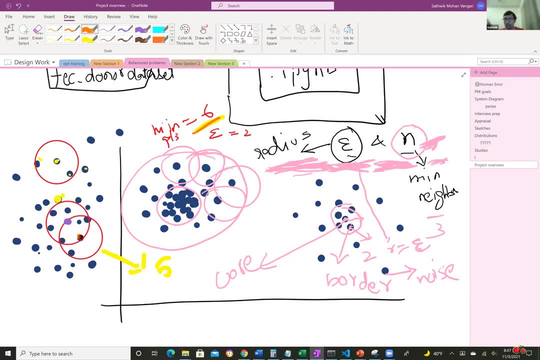 Yeah, to some extent. Again, to some extent, No. I understand. I understand My. my question is: Yes, Everything will have their own circle, though. Yep, Yes, Every single dot that we're looking at will have their own circle. 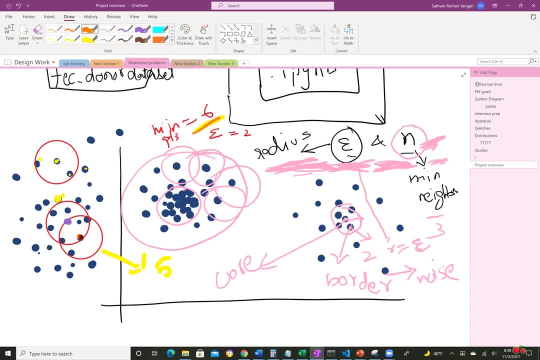 Yeah, they'll have their own neighborhood Gotcha. It just depends on whichever circle you're looking at to determine if it's a border point or a core point or whatever. it is Correct. But then again, see, think of so it's not okay. Let's say okay, this point. 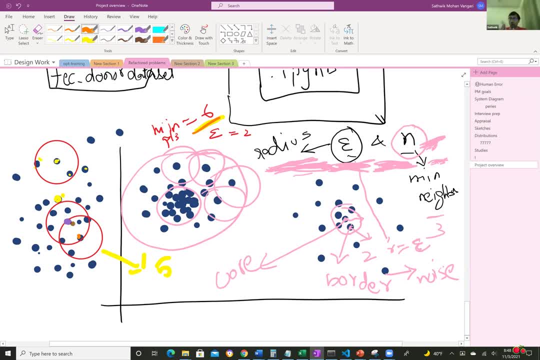 just because it's the center. So every point when you're talking about these circles, right, Because it's at the center of the circle, it's not a core point, or because it's lying on the edge of. so let's say, for example, right, What I'm trying to say here is you. 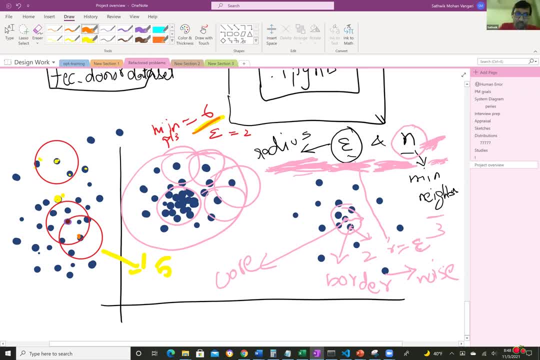 see this orange point right Now with respect to the purple point, this orange point is not the border point, Right. And when you say, okay, when you look at the other circle, right, You are not saying that, oh, this is a core point because it's at the center of the circle. That's not the 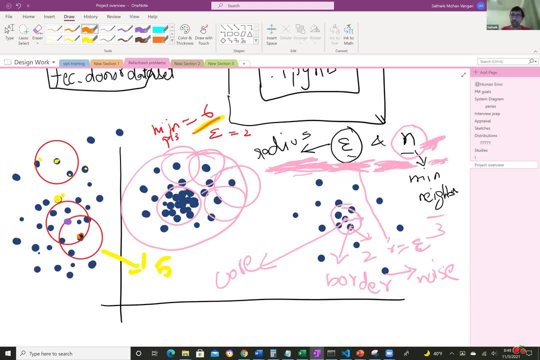 concept here, Right, Okay, The concept is: these circles are just drawn to show, to visualize to you guys what it means, what a neighborhood means. Okay, In reality, no, circles are drawn. These are not the borders that are being checked. I'll tell you. I'll tell you exactly what I mean. 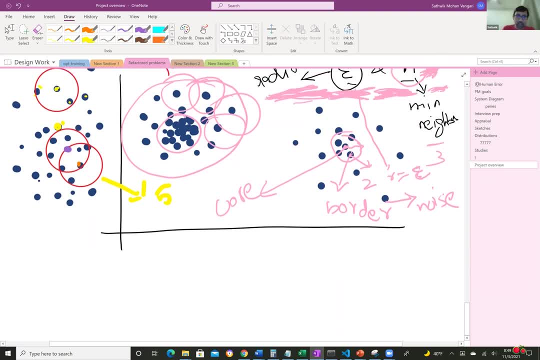 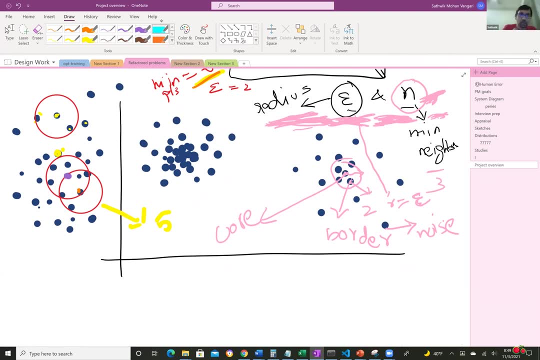 Okay, Now, if you see this right, if you see this, can you all tell me, can you all tell me where the core, the density of the structure is, Where there's more density of the circle, of the points right in the middle, right? 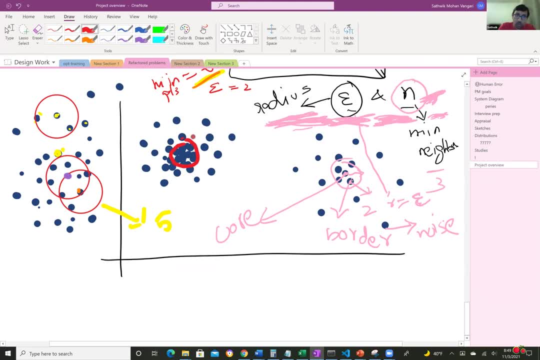 This one right here, Right now. if you see these points all around, right, Okay, Let me mark them in a different color. Let me get these points. that's right in the right dead center. Okay, Now let's talk about these points. 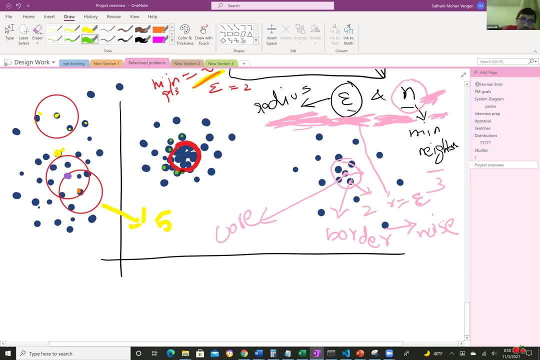 Okay, These are the points with the green dots in them. Okay, Now, what do these points with the green dots in them look like? Don't they look like the border of the center of the core, where there's too much density? right, Now, you guys understand, right, These points. 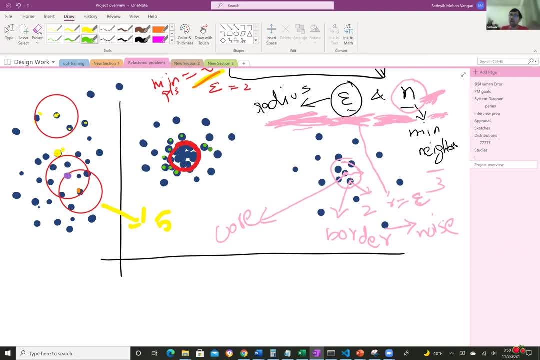 right in the dead center, within the red circle that I draw. they will become core points because they are very tightly packed to each other And most of them will satisfy this condition right, That they will have at least six points around the circle of, say, two units. 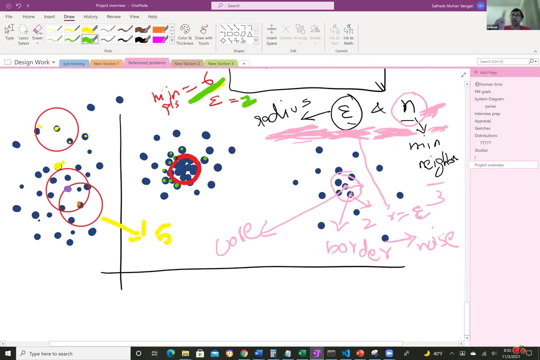 when I draw right, Most of these points will have at least six neighbors around them. The border points may not have six points around them, but they are in the vicinity of core points And so they become the border points. They are still what you called as the outer. 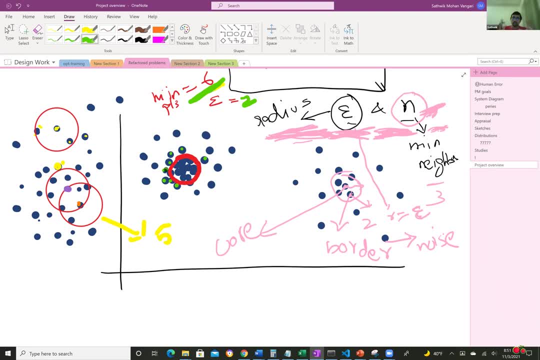 edge of a dense packing right. And all the other points, All these outer points, right Now, you see these points right, They're too far away from the real density. right? That's what you call. this noise Makes sense? No, And that's. 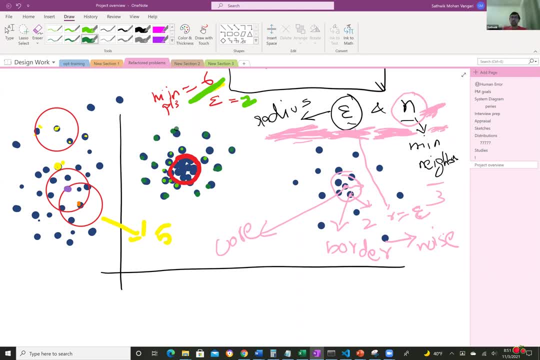 what you're trying to achieve by drawing these circles. Okay, So with that, we're going to draw a circle of six neighbors. So, with that in mind, for this purple point, this purple point will be a core. What do you call? It will be a core point because it satisfies. 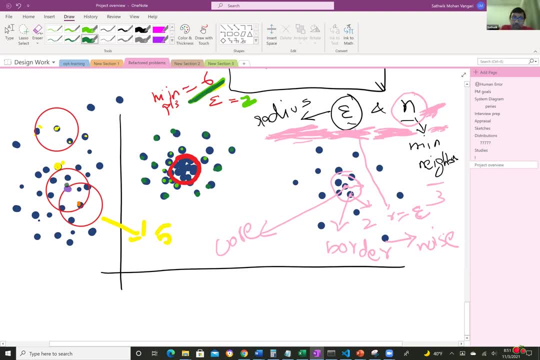 the condition of having at least six neighbors in a circle of radius two around it. right The other orange point. It has less than six number of neighbors in a circle of radius two around it, but it is a neighbor. It is in the neighborhood of the circle, So it's. 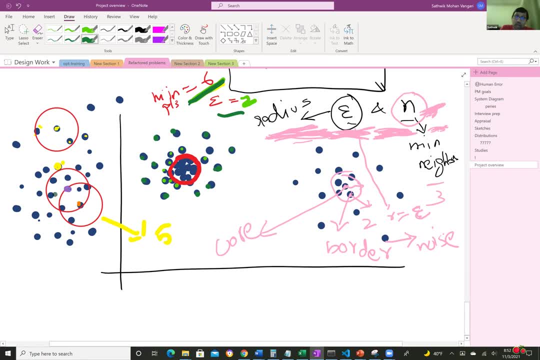 a neighbor. It is in the neighborhood of a point which is marked as a core point. Okay, And that makes it a border point because it's closer to the core point. right, Makes sense now, Okay, cool, Anybody else has any other question? Yeah, So if you call those ones, 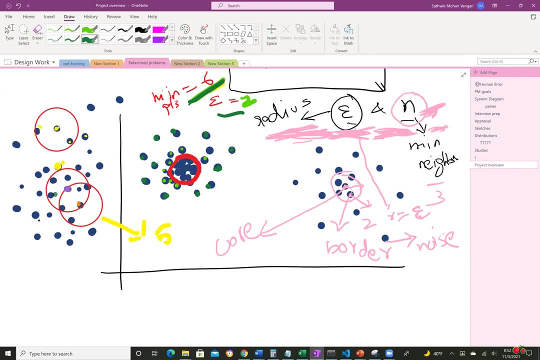 noise? They are not. It's not like they are. Well, you can still draw another circle to get them into like a border point, right? Okay, That's a good question. So you mean to say that you know, okay, I will draw a circle around this point, this point as well, You will draw. 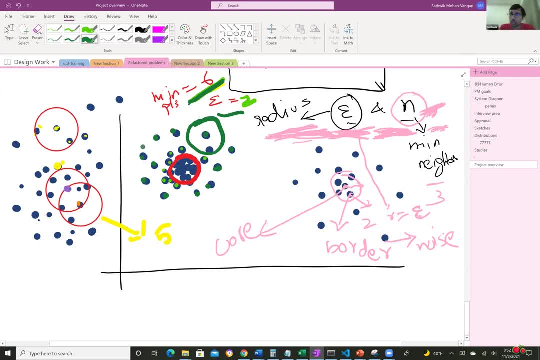 and that's how they are identified as noise. So you draw a circle around every point. You don't leave any point, right? But when I draw a circle around this point as well, and that's how I mark it as a noise in the first place, right? So I draw a circle around this point. 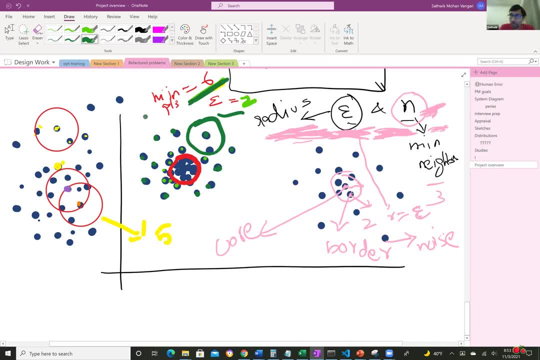 but I don't have the minimum number of points, minimum number of neighbors, which is six. I don't have six neighbors. This point doesn't have six neighbors, right? Let's say, let's call this point A. Okay, Now, A doesn't have six neighbors And is A a neighbor of a border. 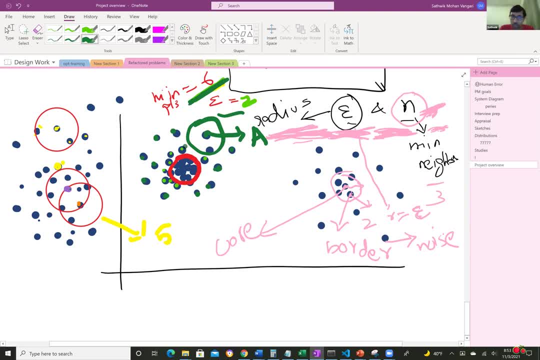 point. No, right, It's not a neighbor of. let's say this point right. Is it a border point? No, because it's not a neighbor, It's in turn. it is not a neighbor of a core point. 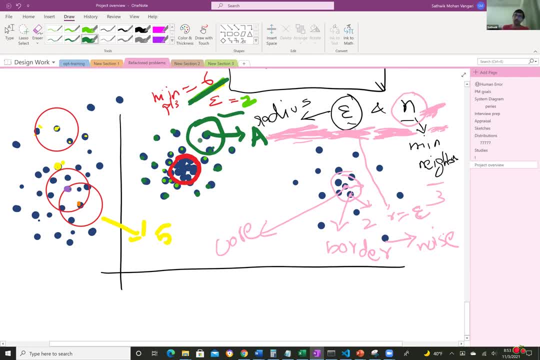 Right. A border point is a neighbor of core point, A noise point is a neighbor of nothing, right? Basically, it doesn't satisfy both conditions, which is minimum number of neighbors and being in the vicinity of a core point or a border point Make sense, I think you. 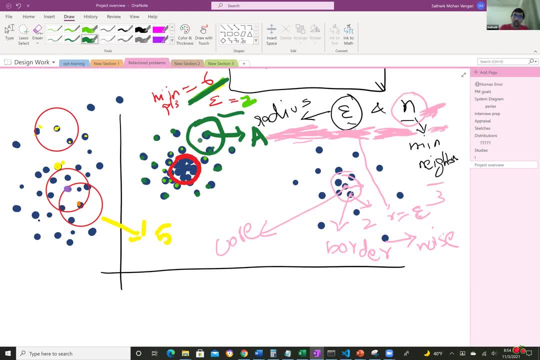 guys, you, you'll get this into your head Once you start Reading up about it. Okay, Make sense, All right, So, and that's how the thing. basically, the DB scan works. right For every point, things are checked. Now, if you have to think about, you know, the application standpoint. 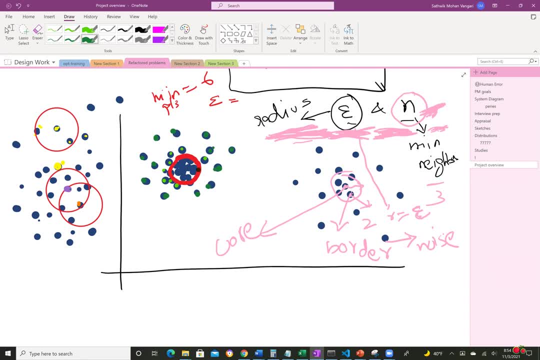 right? Like if you have to visualize something now, think about this as a city, and then let's say: this is a city and there are. these are like houses in a city, right? So if you have to classify a specific area as highly populated, or if you have to classify a specific area, 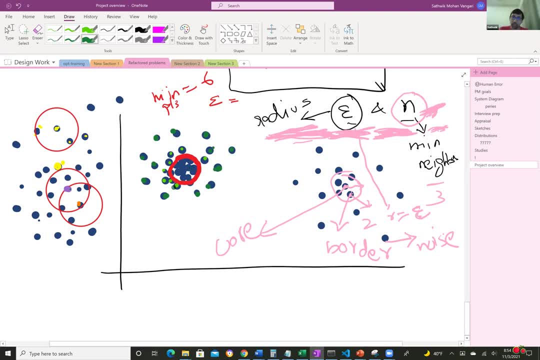 as you know, a community or something like that. think of this as, like my downtown area or something like that, where there is, like two dense, a lot of density of in terms of, like the buildings and infrastructure that's there. The red circle, the borders, is basically the edge of the city and, whatever you see, the 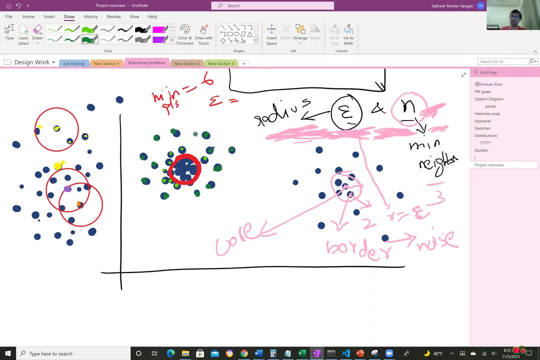 noise that you see all around is basically the outskirts. the suburbs are like the outskirts. where there are are the remote areas, where there are fewer houses or fewer man-made structures of constructions. right, They are, they are scattered around. Okay, Make sense, Can you? 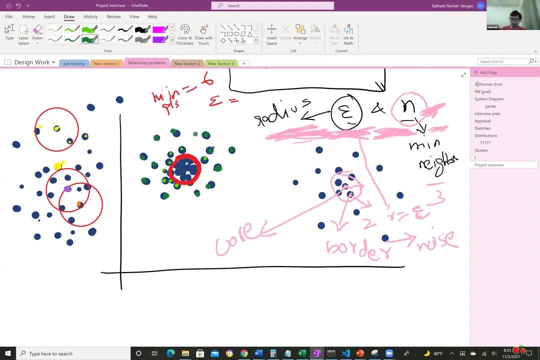 guys visualize that. So dbscan, like, draws a bunch of circles to determine which ones are the core and border points and the noise Correct, and the core and noise, core and border is what makes up a cluster. that's what it determines as, hey, this is one cluster, this is another core, another border, this is another. 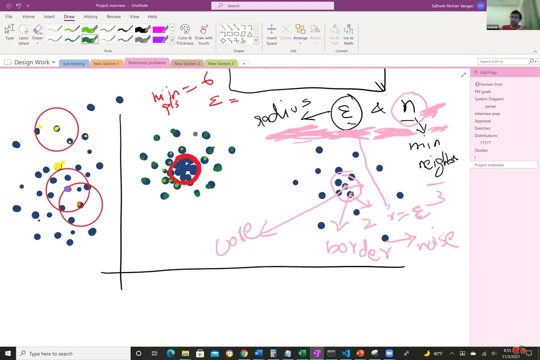 cluster. this is another code, this is another border, this is another cluster. so there are three clusters and the rest of the points which are not belonging to them, which are scattered here and there with a lot of white space around them. no neighborhood, no, not too many neighbors, not too many, not not close to any cluster. that's noise. those are my anomalies. 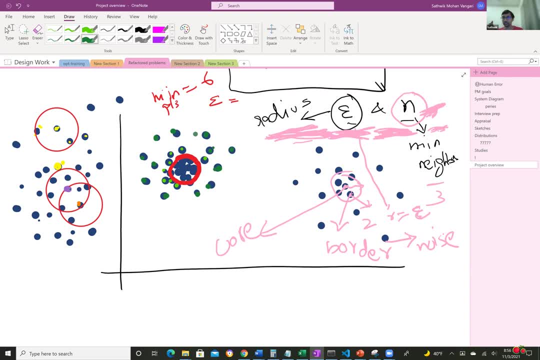 make sense guys. Yeah, I think so Cool, awesome, all right. so in last class I was mentioning about, like, how do you measure the accuracy of dbscan? cellulose score is one metric, as I kind of mentioned, right like silly score, even elbow method. you could use elbow method as well. it's the same as k meets, but and it works. 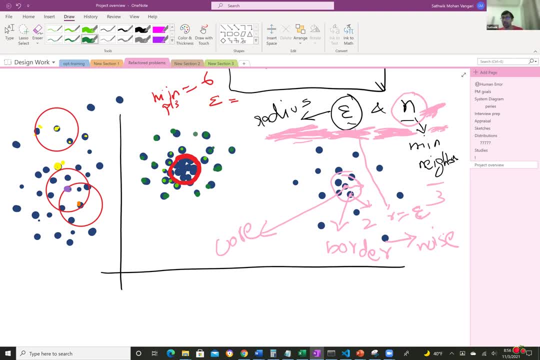 because it's basically looking at the packing of the cluster itself. it both the methods- right elbow method and cellulose score. both of them basically calculate the distance between points in a cluster, right. so if your dbscan returns, say, five clusters And that's wrong, the cellulose score is going to be bad for that. if it returns three clusters. 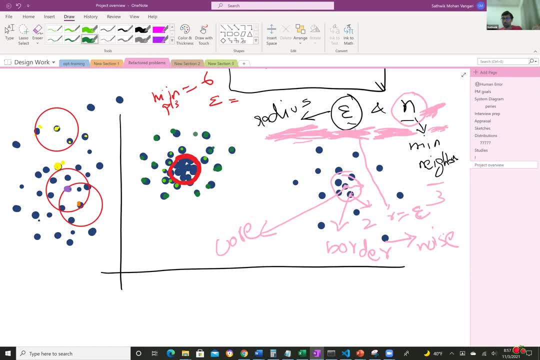 the cellulose score is going to be like. you know better for that maybe, or maybe worse or whatever. right, that kind of tells you what is the optimal number of clusters. So in case of dbscan you don't vary the value k right for k means. it was pretty straightforward. 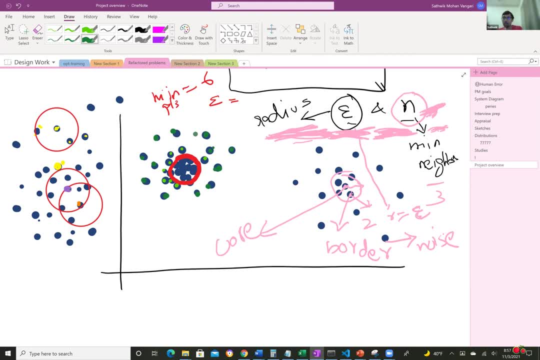 you. So what with k? you said two to ten, two to eleven or two to ten. you iterated between various number of clusters and you looked at the cellulose score. here what you do is you vary these two parameters. you vary number of neighbor, of number of points in the neighborhood. 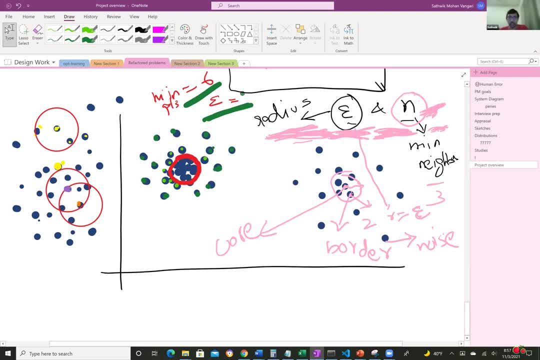 and the size of the circle. right now, in this case, right, I drew a circle. the size of the circle was: what was the size of my circle? this circle two, right, Number two. so let's say if, what if the circle was bigger? say three. now if I put this big. 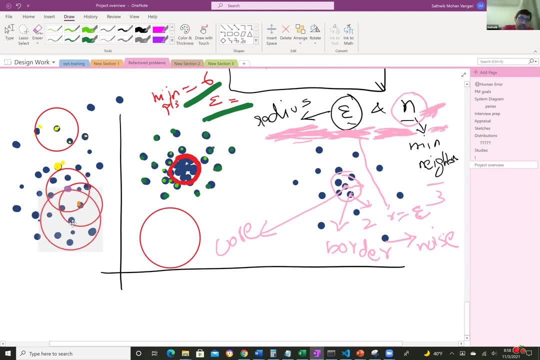 circle around. what am I going to achieve, right? So, if you see, a lot more points will be added to the cluster right. the smaller the circle, the more close the points are expected to be right, the bigger your circle, the more points you can add to your code or add to your cluster right, even such a, you know, basically such: 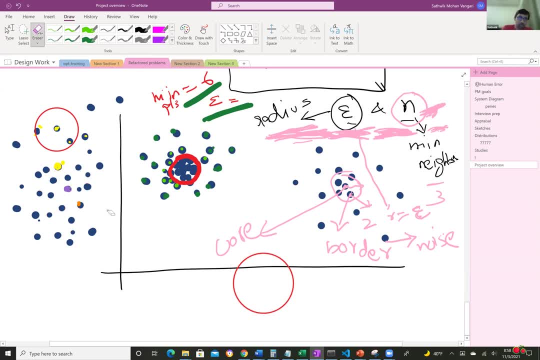 a distribution can also have. let's say, if it's a big circle, right, you will probably add a lot more points. if it's a tiny circle, then a lot of points will not meet your criteria. you can vary this as well. you can say two points or three points or whatever, right. 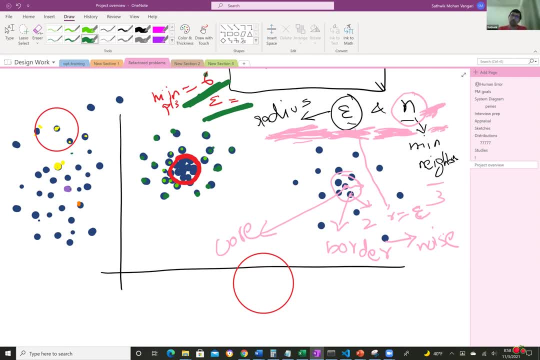 So, based on how you vary these two points, right? Okay, Based on these two parameters, you can create smaller circles and have a lesser number of neighbors. you can say only one neighbor is needed, or you can create a big circle and say ten neighbors are needed. right, because I'm having a big circle, so you can vary both. 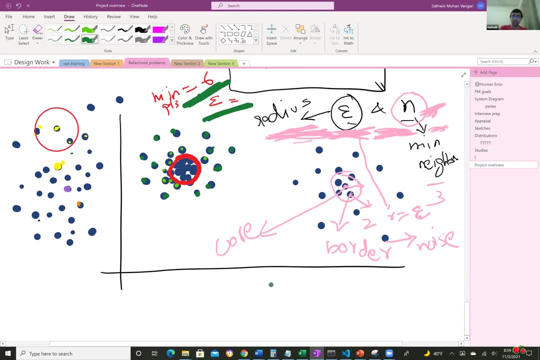 these parameters- the number of neighbors, the number of points, the size of the circle- and based on that you build your clusters right. and that is where the difference comes. when you vary these two parameters, You might end up with three clusters, four clusters, five clusters, six clusters, depending. 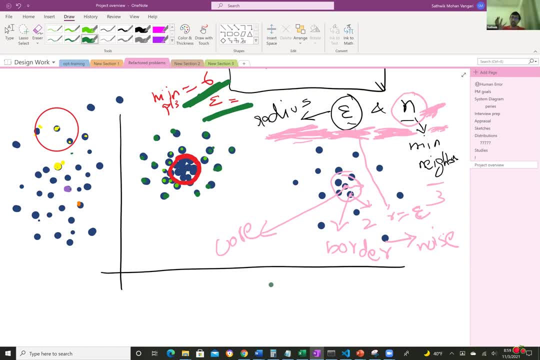 upon what you set up as the number of neighbors and the size of the circle, you might end up with different number of clusters and that's how your silhouette score result will also keep changing right and as and when you your silhouette score changes, you keep a track. 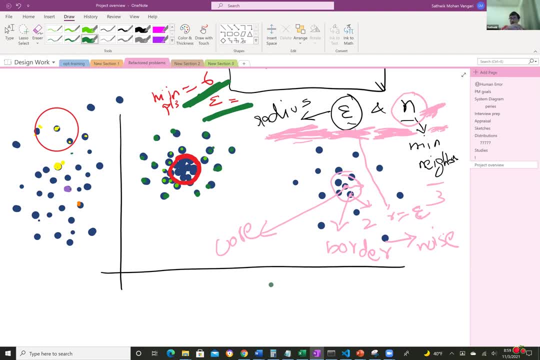 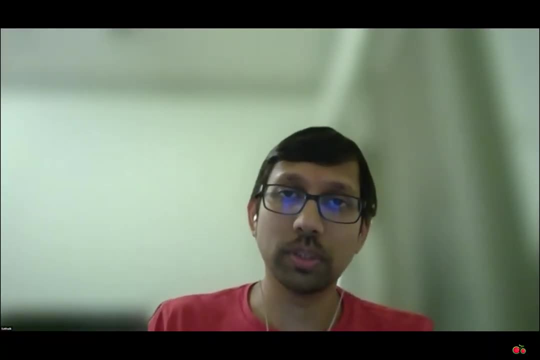 of it and wherever it peaks. if it's a loose score, wherever it peaks, that's your optimal number of clusters. if it's a elbow method, wherever it bottoms out- the tip of the bottoming out Aspect, that becomes the number of optimal clusters. so far, what we studied in unsupervised- 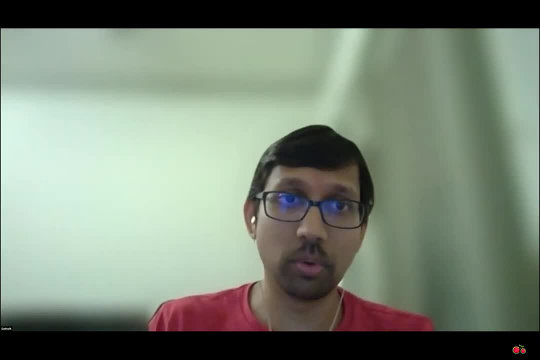 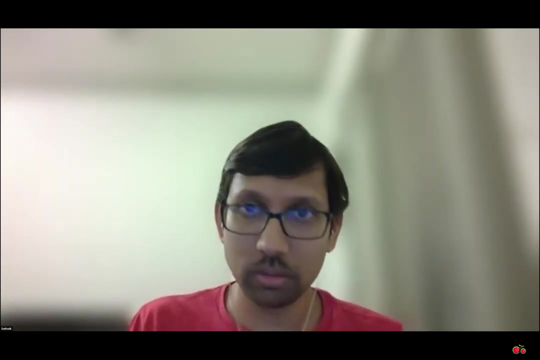 learning at least the first half of this class, couple of classes before k-means db scan. these are clustering methods under the unsupervised learning right. what does that mean? basically, the we are, what are you, what do you do in clustering? can anyone tell me what's the goal? 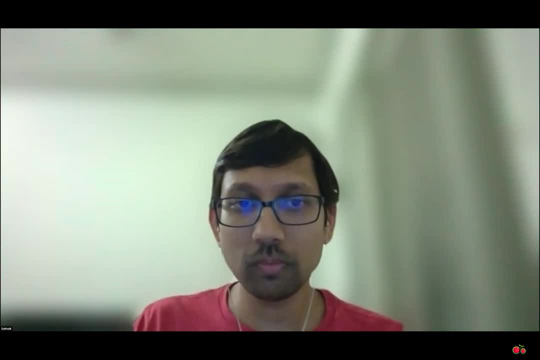 what are you trying to do? Trying to group, like data? yep, so you're basically trying to, you know, understand the underlying structure of your data, group them, you know, group similar points or similar observations together so that you can apply similar inferences to that group of people or observations, or, 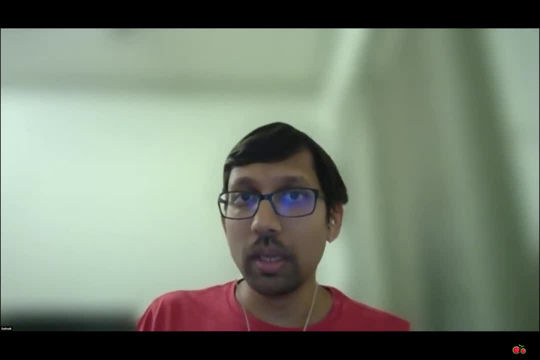 whatever right, That's what you're trying to do With clustering. now there's the other type of unsupervised learning technique, which is called as dimensionality reduction. okay, so, and that's what is. that's what we're going to discuss about today, and that's what principal component analysis is all about. okay, just. 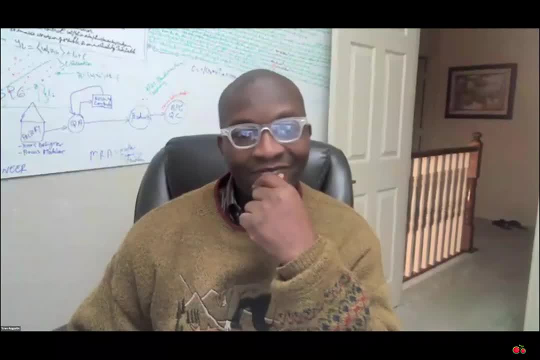 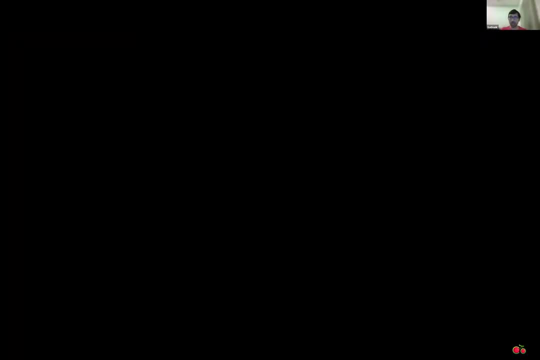 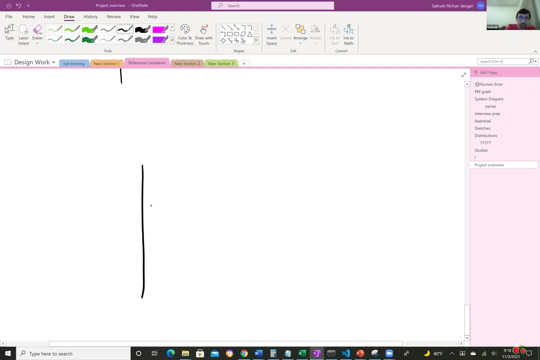 give me one second, all right, so let me quickly share my screen. yeah, Okay, Okay. So let's say: you have a table, your data right and you have right. so this is one, two, three, four, five, six, seven, eight, nine, let's say okay. 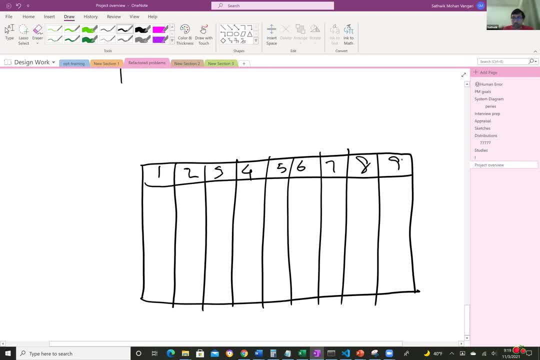 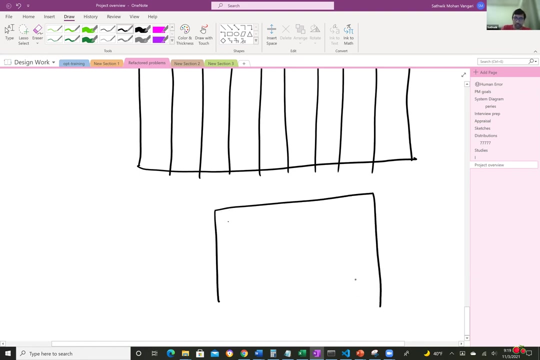 Okay, And so you have about nine columns in this data set, right? so what do you get when you do a correlation plot? so, by the way, why do you do a correlation plot? You guys remember correlation plot, right? correlation matrix From ds2. can anyone explain? 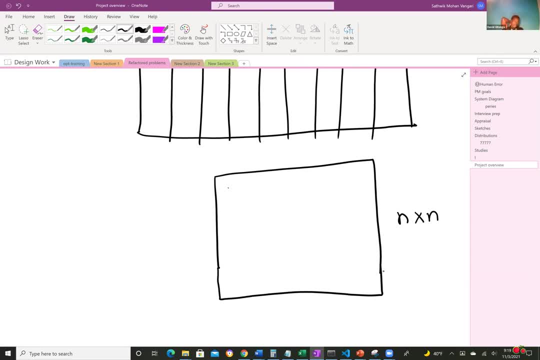 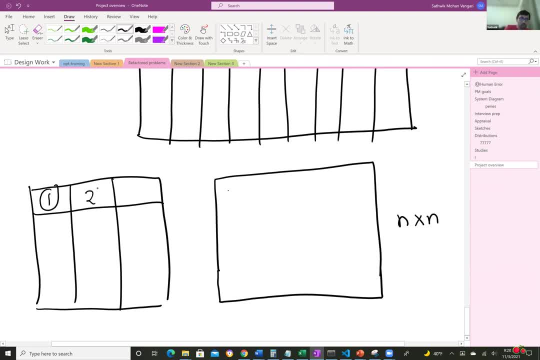 Okay, Okay, Okay, Okay, Okay, Okay. Any guesses. why do you do that, guys? why do you draw a correlation plot, You know, to determine which ones Which Which columns will be able to fit in into the model. All right, 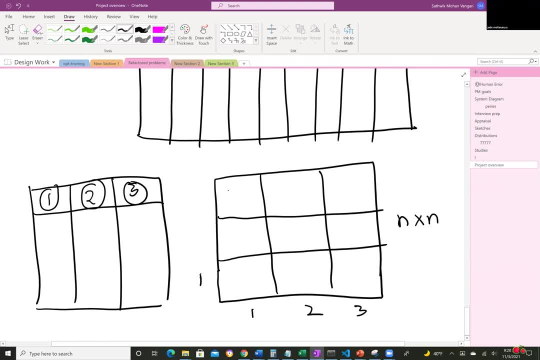 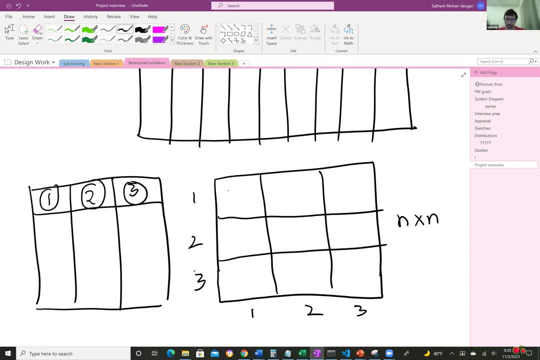 uh, which ones are independent of each other right now? why is this important? so let me, let me tell you that, let me get to tell you guys that. so let's say we are trying to predict, um, the- let's take that example of the shirt- right, the price of shirt using a couple. 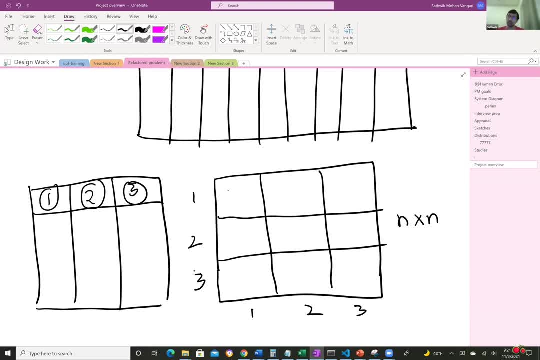 of components. right, we use the cost of cotton, we use cost of labor and then we use cost of equipment. right? so these are three components: cost of cotton, cost of labor, cost of equipment as three components. right, so we use cost of labor as three components. right, so we use cost of. 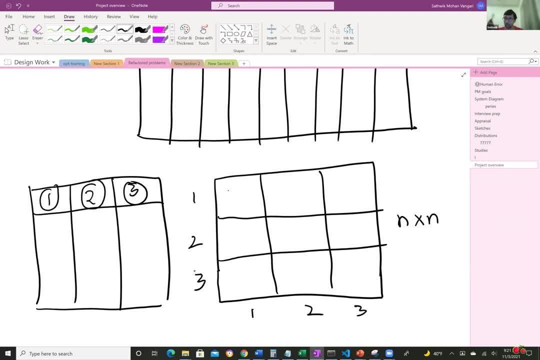 labor as three components. right, so we use cost of labor as three components. right, so we use cost of three predictors for the price of my shirt right now. does cost of cotton depend upon the cost of labor? think about it and answer what do you guys think? yeah, so it does. yeah, okay, why do you think? 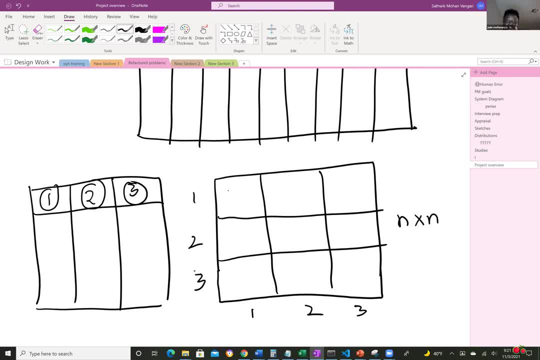 wait. cost of labor? yeah, cost, of course. cost of cotton. cost of cotton, right, the cotton, the material that you're buying to sue your shirt, right? oh no, they won't affect this, right? uh, what? what do you guys, other guys- think what? what do others think cost of cotton and cost of labor are? 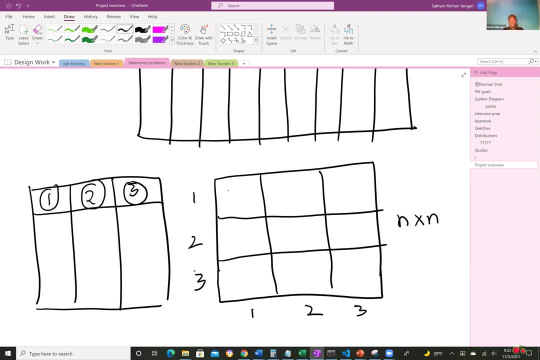 they related. do you think that if the price of tomorrow, the price of cotton, goes up immediately, the laborers will demand more money? no, no, right, so they're not related in any way. exactly so they can be related in africa, because anything that goes off, everything goes off. 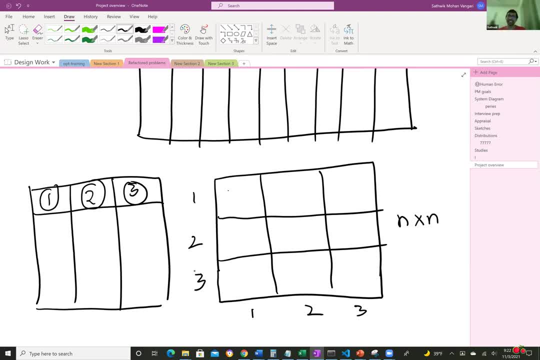 so well, that's a see, that's a um, that's very situational, and see, that is something is called as spurious correlation. okay, there might not be a direct link between both of them, right? um, it's not mandatory that one is linked to the other, it's just that people are basing their own. 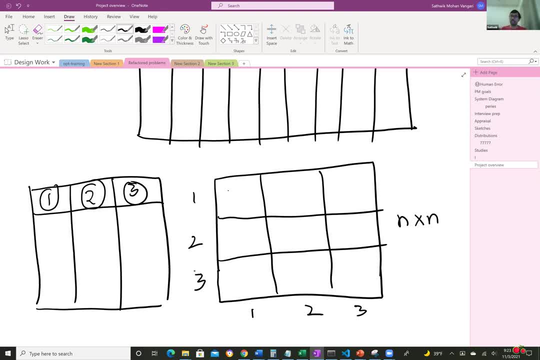 basing their perception off of the you know other aspect. but, um, usually that's not how things work, so there's something called a spurious correlation read up about. it is pretty fun, okay. so cost of cotton. let's assume this is cost of cotton, right, this is cost of labor. okay, let's see. 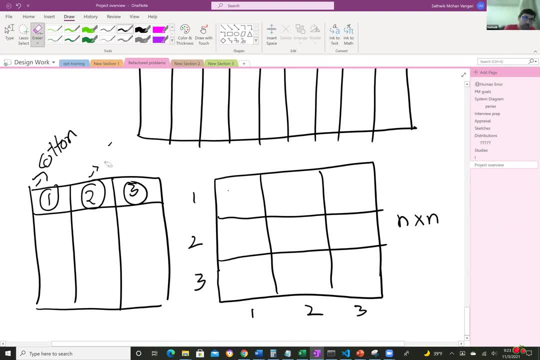 cotton. labor and equipment. okay now. do you think that labor and equipment are related? what do you guys think? labor and equipment? i don't think so. what do you think? david jude eve's? what do you guys think So? which one? labor and equipment? Labor and equipment- yes. 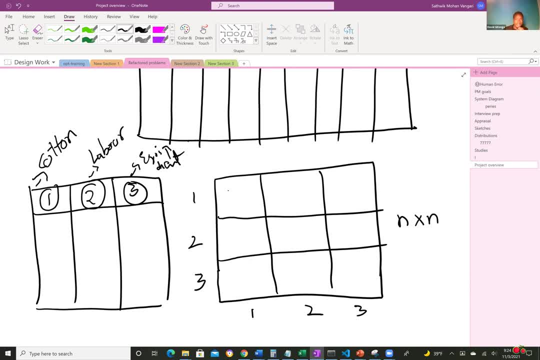 They are not related. Not related, They are not Okay. Maybe they are related Or maybe Why. If it's specific equipment that only some people can operate, yes, Okay, That's a good justification. What's another justification? 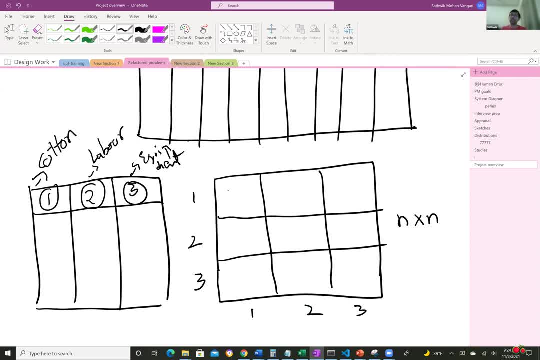 The more expensive your equipment, the less your people might have to do, Which means that, let's say it's a machine that takes in the cotton and just gives out a shirt, You'll probably need only one person to monitor it. You don't have too many people who are looking at things. 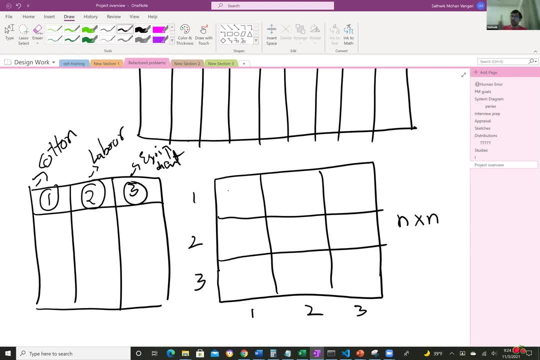 If it's a machine that's doing everything by itself, But if it's a machine that is only filtering your cotton, you still need labor to sew the cotton into a shirt. So, depending upon how expensive the machinery is and what parts of your operation, 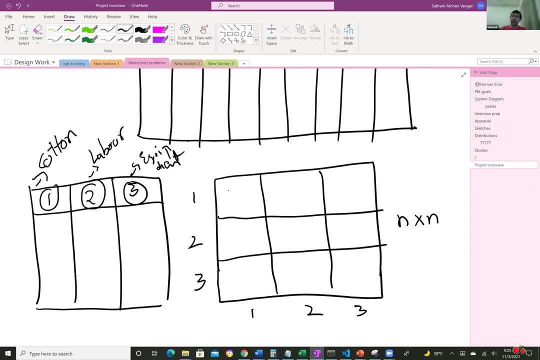 it is taking care of your labor and equipment cost might be related, But again not as strongly, It's weakly related but it might be related. So the coefficient of correlation: it ranges from minus one to zero to plus one. 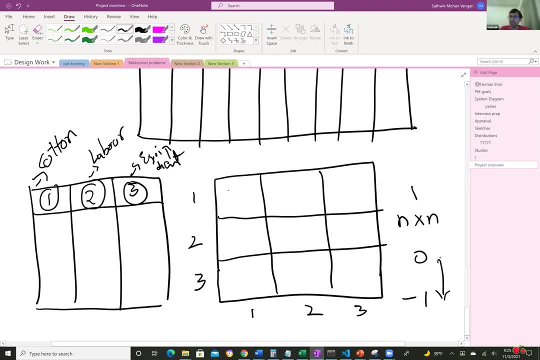 So minus one to zero basically means that it's negative correlation, Which means that if one thing goes up, the other goes down. So, for example, let's assume for a moment that labor and equipment are slightly correlated, Which means that if I buy equipment which is much more expensive, if I'm putting a lot of money on 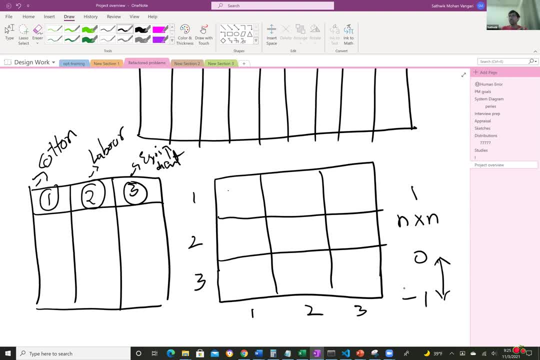 my equipment. Buying much more expensive equipment which is taking care of some of the operations, I can fire some labor and instead get that work done by my advanced, sophisticated machinery. So what happened here? my cost of equipment went up and my cost of labor went down. 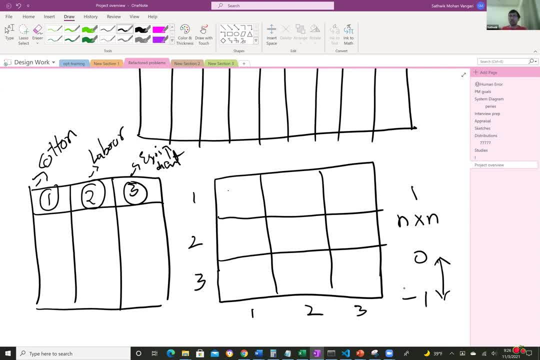 Or let's assume that I had very sophisticated equipment, but I thought, okay, let me get rid of it and buy simpler equipment. But now I need more people in order to take care of the things that the machine is not doing, the machines might not do. I gave up the sophisticated equipment. 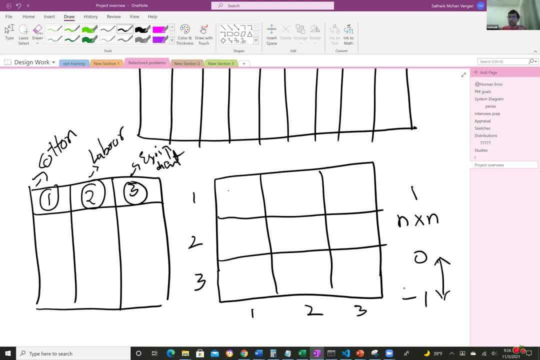 So cost of equipment went down, cost of labor went up. So you see the idea: One thing goes down, the other thing goes up. Now, if this is the case, if they are related, if labor and equipment costs are related, and if one thing goes up and the other, 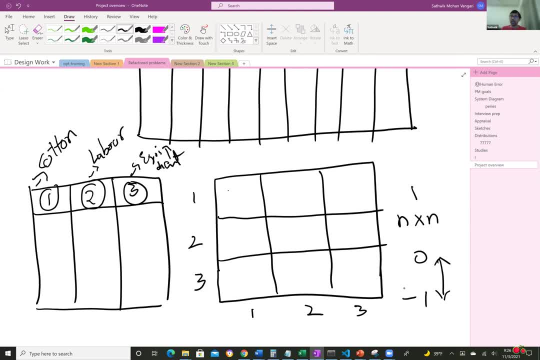 thing goes down, it's negative correlation. right, They are inversely proportional. If you guys remember proportionality, we call them as inversely proportional or negative correlation, right, One thing goes up, the other goes down. So that will give you a coefficient. 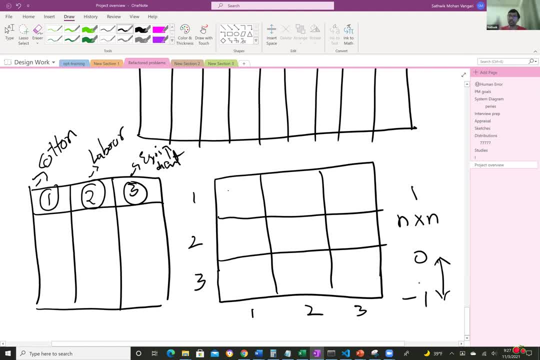 somewhere between zero and minus one. It will be a negative value right Now. what is positive correlation? If one thing goes up, the other also goes up. right, Let's say, for example, the type of cotton. right, Let's say: I am using high-grade cotton. right, And only high-grade. 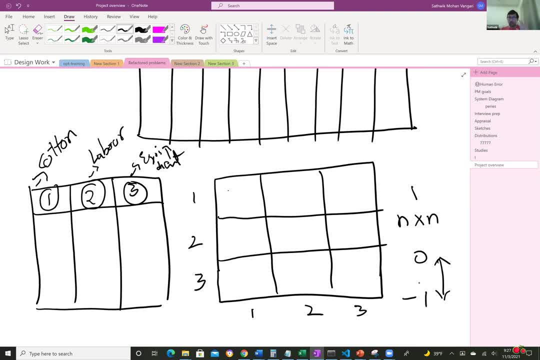 machinery or equipment can process that cotton right, Appropriately right. If I put high-grade cotton in cheaper machines right, They might actually be tearing that cotton away, or they're not able to process that High-grade cotton appropriately right, So the high-grade cotton is more expensive Low-grade. 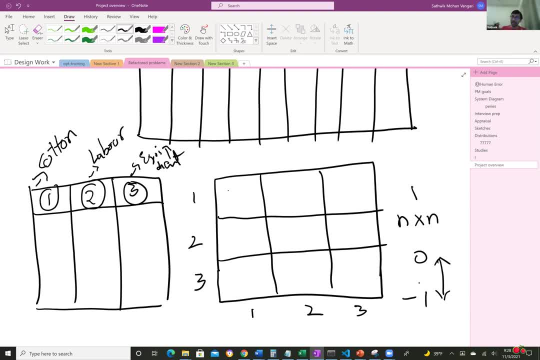 cotton is not expensive, Low-grade cotton. if I put it in a highly sophisticated machinery right, The machinery might not work well with it because of the impurities in the cotton, like the seeds being left out, it not being bleached or all this kind of various aspects. 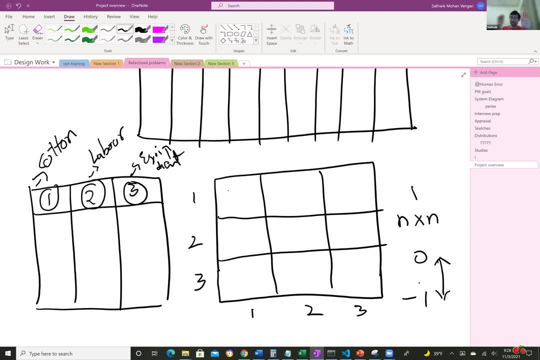 of the low-grade cotton right. Let's say, high-grade cotton requires sophisticated equipment to process. Low-grade cotton can work on lower, It can really do the job. if it is presumably hard to have overhard quality They can work on singing Contra- same as low-grade machine. But if I have a top that can't process any, 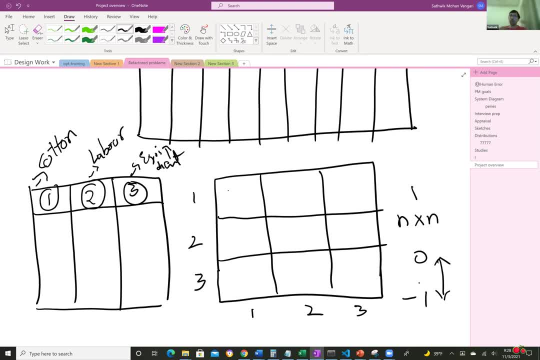 of that sort of high-grade machinery. Neither of them can fit, uh, the lower category, right? High-grade can't be processed on low-grade equipment. Low-grade cotton can't be processed on sophisticated or high-grade equipment, right, In that case, if the cost of cotton 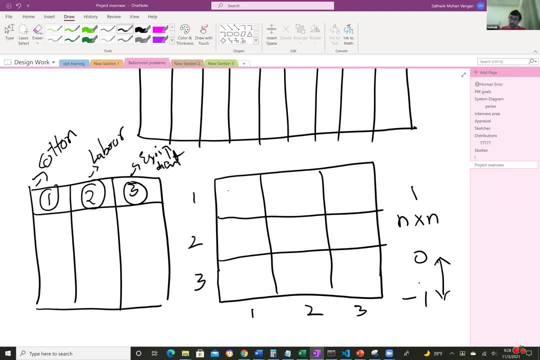 goes up If I am, Instead of using cheaper cotton, I'm using higher priced cotton, Right, The price of my equipment process it right now. this is positive correlation, right, so the value of your correlation coefficient will be between 0 and plus 1 in that case. you guys are understanding, both increasing. 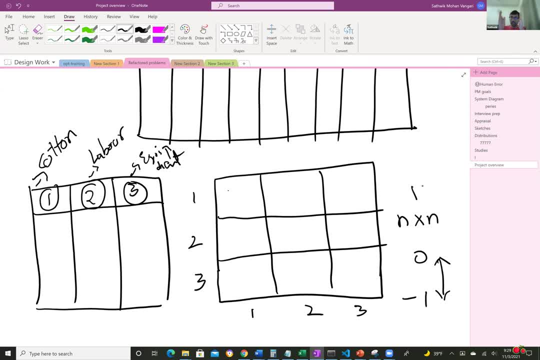 so one variable increases, the other also increases simultaneously. that means that both of them are positively correlated, or both. one decreases, the other decreases. both are positively correlated if one decreases, the other increases. if one increases, the other decreases. right, the opposite is happening. then it is negative correlation. clear guys. 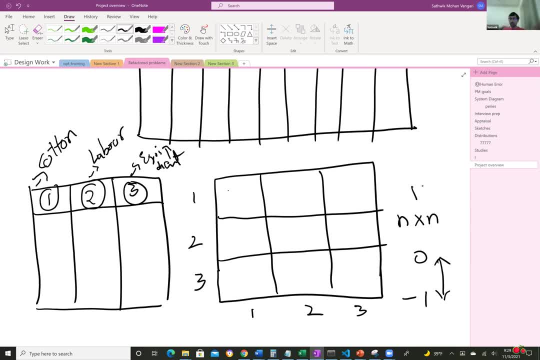 understood. now, when do you say there is no correlation, when increase or decrease of one element does not affect the other one? absolutely, that's perfect. that's a perfect answer list. so, and that's what exactly happens with cotton and labor right, increase or rise in price of my cotton doesn't affect my labor cost or decrease in price. 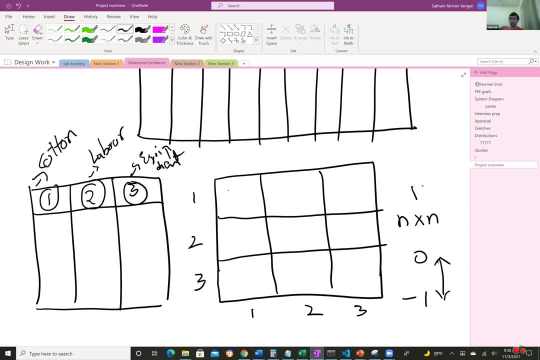 of cotton doesn't affect my labor cost, right? so if we have to, if we plot, uh, if, based on the assumptions that we just discussed, right, if we plot our correlation matrix, right, how does it look like? first one is cotton, so this one will have uh red color. let's say, one is red, this is white, right, and this is blue. 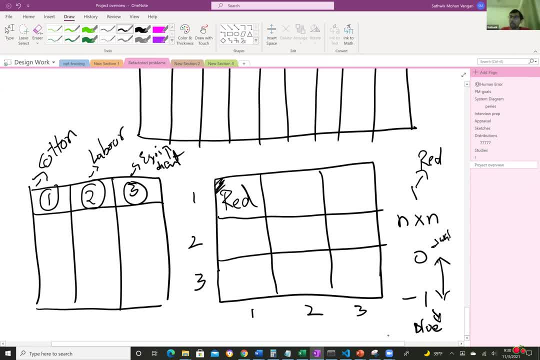 right and the numbers basically tell me that. so, from white to red, the more red the color is, the higher the number, okay. the more blue the color is, the lower the number, okay. so this one will be red, this will be red and this will be red. why? because a variable is always positively, perfectly positively correlated with itself. 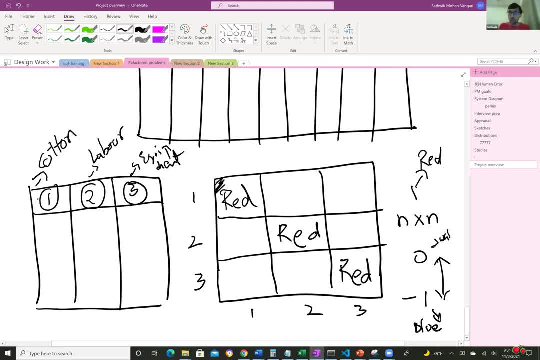 right, obviously, if i'm considering cotton and if i have another column of cotton besides it. right. if price of my cotton for one pound is two dollars, the second column will also have two units. uh, in in that row, right. second day: if price of cotton has gone to three, is the same column right same. 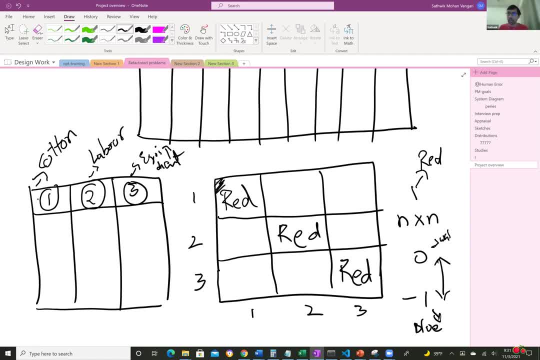 value. so three, three, four, four, five, five, six, six right. three, three, four, four, five, five, six right, or one, one, point five, point five. so it'll either decrease and increase, the same, with exactly the same magnitude as well, and the same with labor right. let's say, cost of my labor is five dollars. 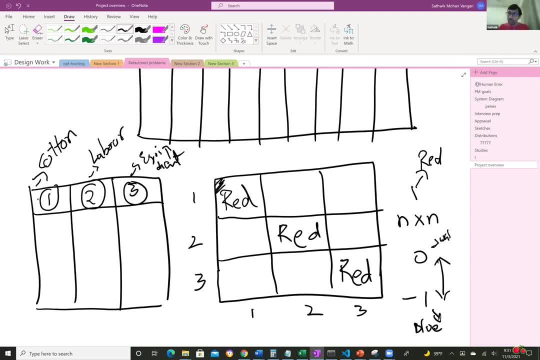 today, tomorrow it's ten dollars. if i have another column of labor besides it, it will be the same value, right? so every column is perfectly positively correlated with itself. so all this, the diagonal right- one, one, two, two, three, three- will always be red, which is perfect, positive. 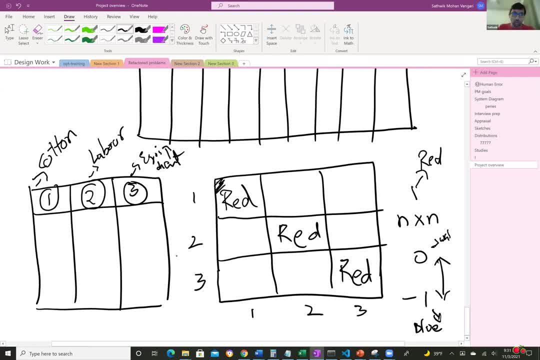 correlation now, but one in correlation with two right, cotton in correlation with labor. what do we think of? it has no correlation, which means, uh, one with two will probably be white, one with two will probably be white right and one with three cotton and equipment. this will be closer to red. 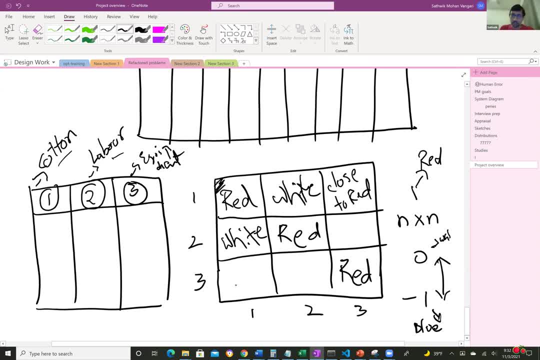 close to red, might not be perfectly red, but close to red, okay. and what do you think? this other thing will be two and three, that is, labor and equipment. what did you discuss? just know what did we discuss? what's the relationship that we assumed that labor and equipment have? 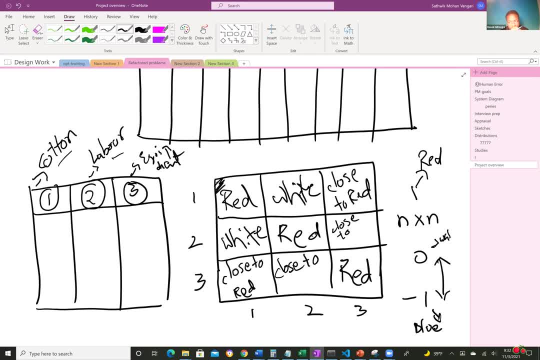 sorry i'm gonna say negative or positive, i don't remember. so did we say was if it could be related. it could be related, so it's a positive right. yeah, assuming it could. they could be related. what did we discuss? if i buy higher priced equipment, what happens to my labor cost? it goes down right, but if i buy cheaper equipment, 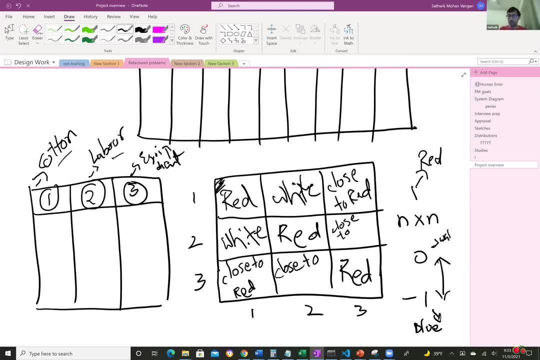 my cost of equipment goes down. what happens to my labor cost? so what correlation is it right close to red? okay, i guess we're using why? why will it be close to red? because the two and two correlate to each other, because it's the same column. yeah, two and two, but here we're. 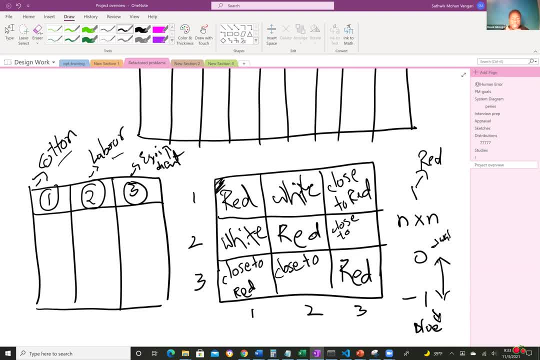 talking about two and three: right, labor and equipment. yeah, so i'm assuming red means closest or, you know, directly correlated to each other. so if, if, positively correlated, yeah, positive, positive and negative. is this positive correlation, although, because cost of equipment goes up, labor cost goes down? what is positive correlation? 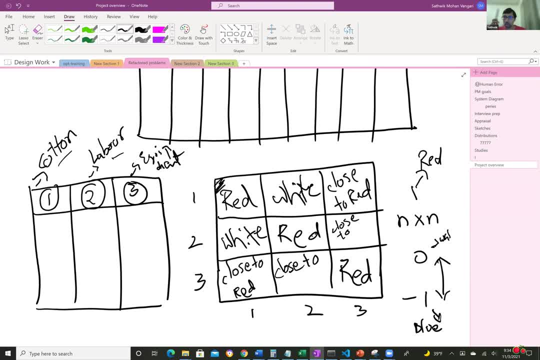 cost goes up, labor cost goes up, cotton cost goes up, or cotton cost goes up, equipment cost goes up, cotton cost goes down, equipment cost also goes down. that is positive correlation, okay. so it's negative, exactly. so this will be close to blue, i don't know right. yeah, because it's blue. i, i wrote here right, so the minus one will be blue. 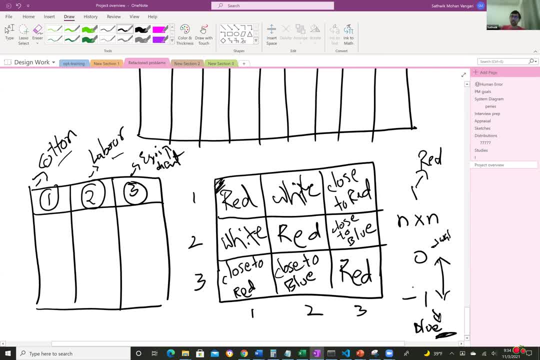 color. so when you draw the correlation plot as well, this is the color scheme that you will have by default. i don't know if you guys remember that from ds2, but on the right side you will see minus one, zero and one. so closest to plus one, the color will be red, completely red. the middle will be white and 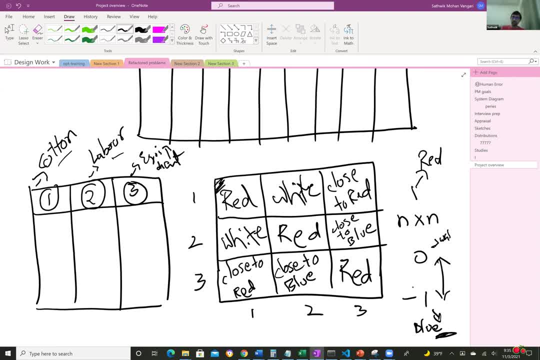 the bottom will be completely blue, right? so these are the colors that you will get when you do a correlation plot. now why did i explain correlation plot so uh? so much to you guys. so if you guys remember, with this correlation plot you can identify which columns might seem related. 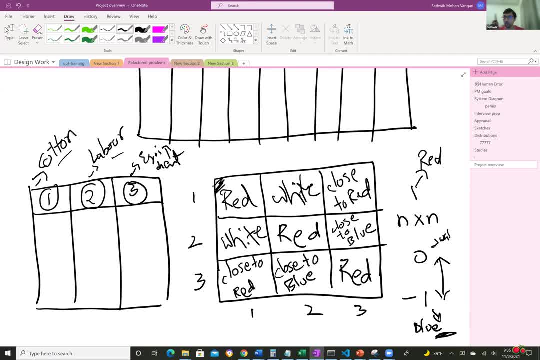 right now, if you see very strong correlation between two points, right then one or the other of those columns might be derived or might be influenced by the other right, in which case- right in this case- the correlation might not be too strong, but let's assume that it is too strong. 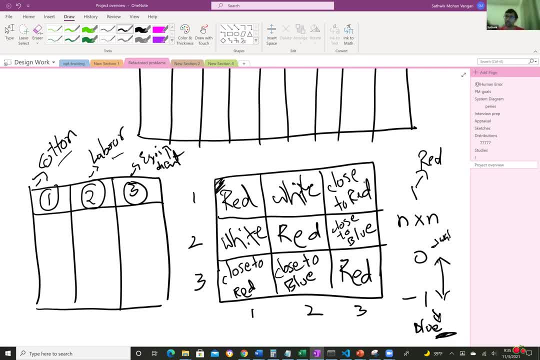 what do you do? you keep one of the variables and you throw away the other one, right? you do not keep highly correlated variables as your predictors. two highly correlated variables as your predictors. why do you do that? because each of these variables have a specific effect on your target. 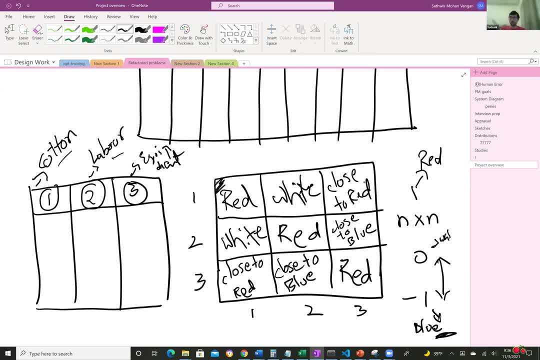 right. and what's my target in this case? price of shirt, right? so let's say, for example, let us look at the labor and equipment cost and let's assume for a moment that they are very high, negatively correlated- okay, so, if it is very highly correlated and if i'm using either labor, 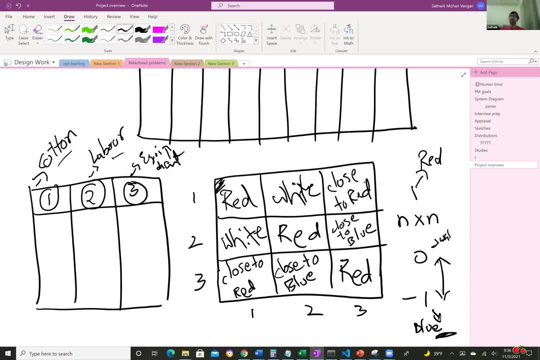 so let's assume it's to the extent that you know, i have one of them as a major cost. that's it right. i either have advanced equipment which is just sewing my shirt and i have very less labor, or i have a lot of labor who are sewing, cleaning the cotton, doing everything by themselves, and i 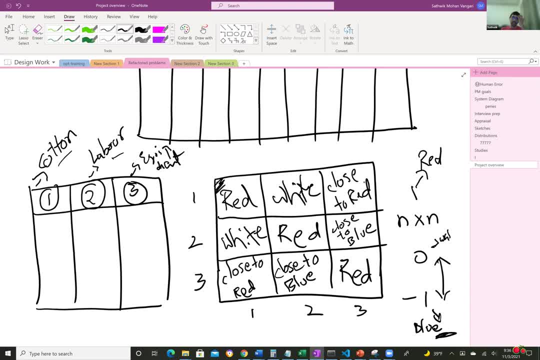 have very minimum equipment, right? these are the two possible scenarios let's assume right now, in effect. so what is really affecting the price of my shirt at the end of the day, right? cotton, yes, that is a factor that will affect my price of shirt. then, if these are the two scenarios that 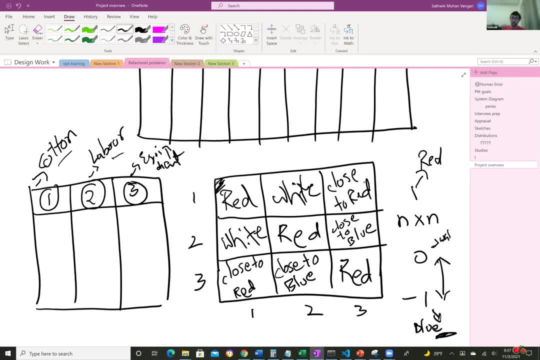 i have posed right cost of either i have high equipment cost or high labor cost. only one of them contributes to the price of my shirt, not both right, because if my labor cost is pretty high, my equipment cost is pretty low and so it doesn't really contribute to my price of shirt if my equipment cost is pretty high and 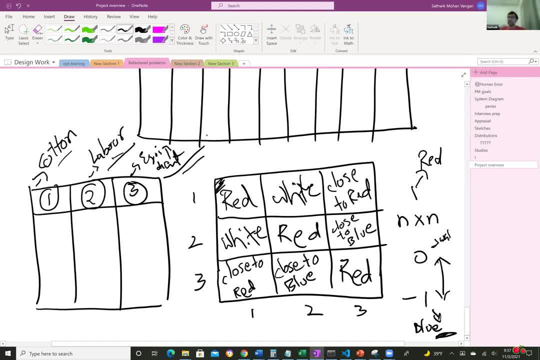 my labor cost is pretty low, then the cost of equipment that i will take into consideration to price my shirt. making sense, folks, right? so it's effect of only one. you know it. if they are derived variables, if they are very close to the price of my shirt, then the cost of my shirt is. 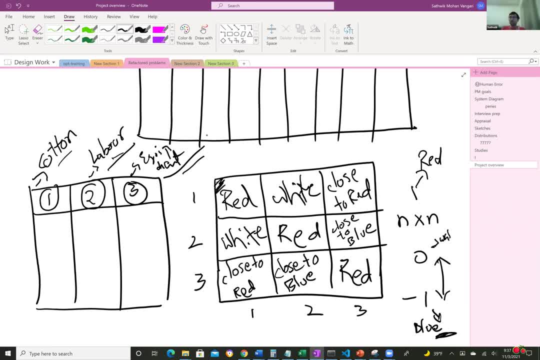 closely related to each other, right? if one variable is derived of the other, if you put both of these correlated variables as predictors in your model, you are doubling the effect, right? you're doubling their effect in terms of the influence they have on the target, right? so you read up about this we'll discuss about in the next class as well, like why this happens. 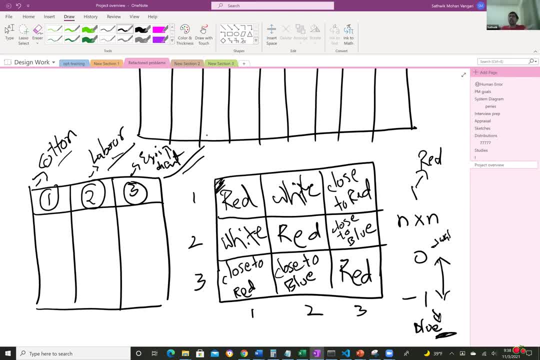 like what's doubling of effect? right, double effect it's, it's a redundancy in data. it's almost like using the labor column twice. or it's almost like using these two columns twice, right, so you don't account for a double effect, right, you account for a single effect. 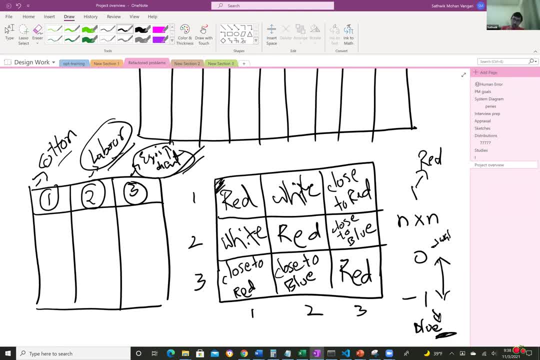 of a specific variable. so that's why you draw the correlation plot. and what you do with the correlation plot is you try to figure out whether there are any correlations or associations between multiple columns and you try to only keep independent columns as predictors in your model. you 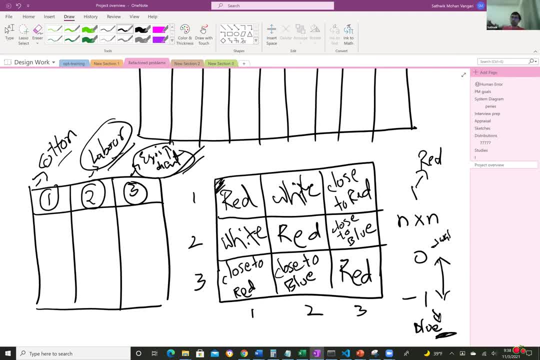 throw out the derived columns. you throw out the columns which are highly correlated to each other because you want to have a single effect or an independent effect on your target variable from a specific source. there are, let's say, three different sources or three different influences on a target variable. you want to just keep three different unique sources rather than having four. 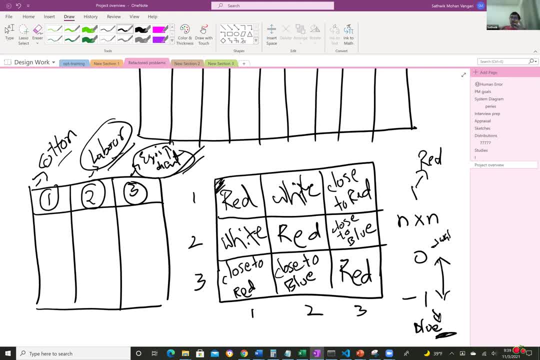 sources, where two of the sources are duplicating a specific effect on the target right, and that's why you use this model and it's a feature selection technique. correlation matrix is a feature selection technique where you try to throw away those columns which are highly correlated right now. this is where it gets interesting, if you have like. here i was taking the example with 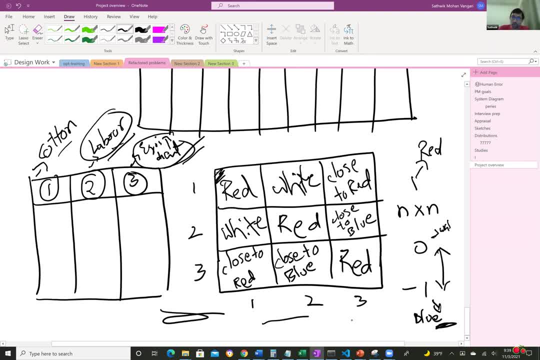 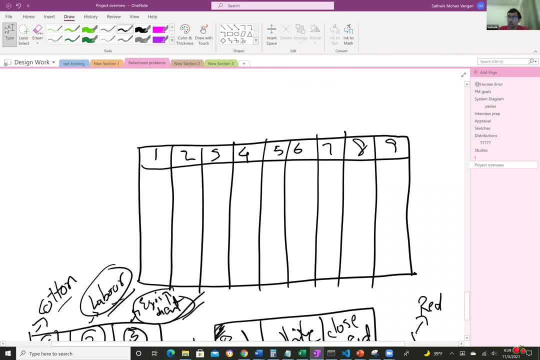 three columns. okay, so i draw a correlation plot and it gives me a three by three matrix right now. what is the correlation plot and what is the correlation matrix and what is the correlation matrix now? as a result of the correlation matrix, if i just half a column, i could draw a three by three. 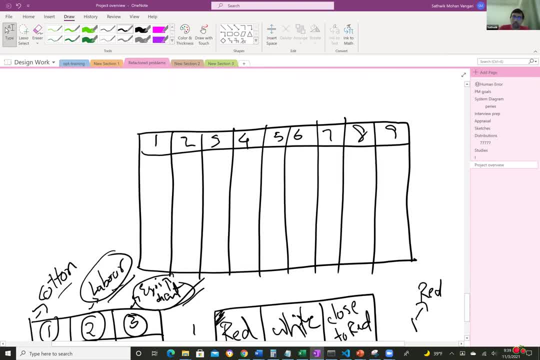 matrix. okay. so what if i have nine columns? how many? what will my correlation matrix look like? it will be a nine by nine matrix right now. okay, that's still probably not that bad, right like. nine by nine basically means that you have 81 cells to look at, but maybe that's not bad. 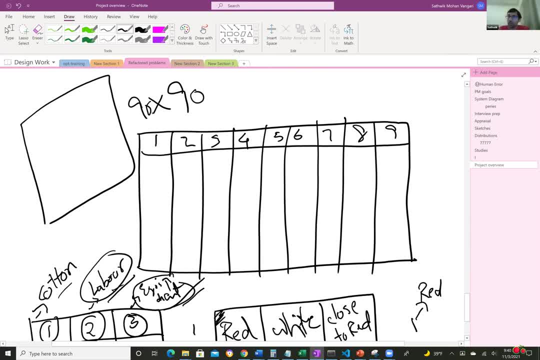 what if you have 90 columns and you draw a correlation plot? can you really select features from a 90 by 90 matrix and then you draw a correlation plot right now? what if i have nine 90 matrix? by looking at the tiny pixels like these blocks, right that you see this red white. 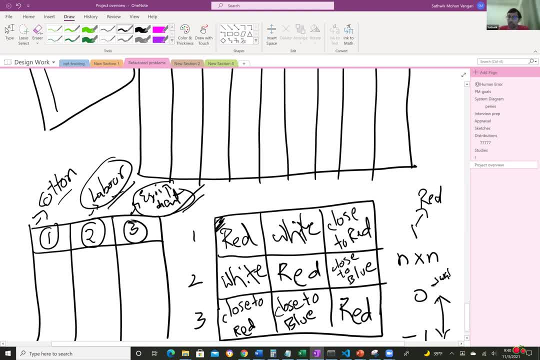 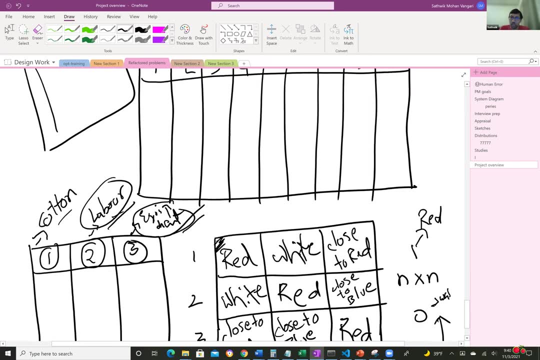 close to blue these colors. you are able to like visually see these colors and like pick out the features because you these blocks are big. now, if it's 90 by 90 matrix, right, it's probably they are going to be 8100 cells in that matrix, right? so each of them will. 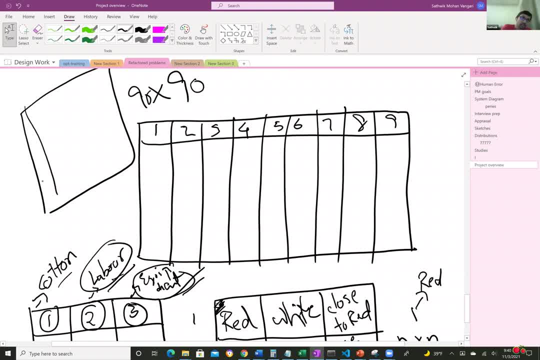 be a very tiny box right, so there will be like so many lines like this right. there is like 90 columns in this and 90 rows in this right, so each block will be very tiny cell. so you can't really with the naked eye right, like when you build this correlation plot. 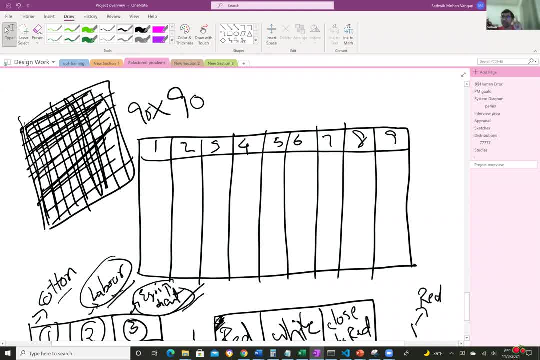 you really can't, with the naked eye, identify. okay, this column should be there, this shouldn't be there. like it's impossible for you to process the entire matrix in a manual way and then decide what features should be there, what features shouldn't be there. and this is where principal. 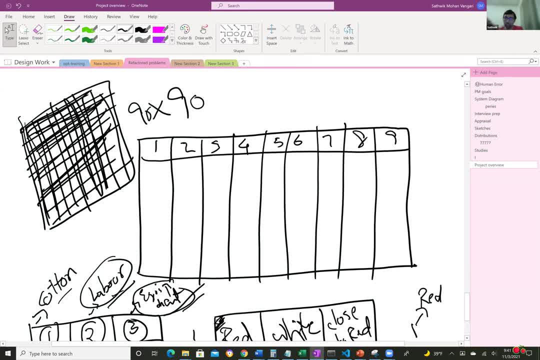 component analysis comes into picture, and that's why it's an extremely important technique i want you guys to like. really pay attention. we will discuss this in the next class as well. we will do a review of it, so don't worry, but pay attention. so all right. so what exactly? 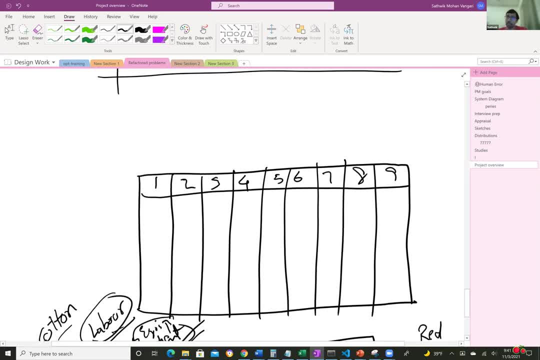 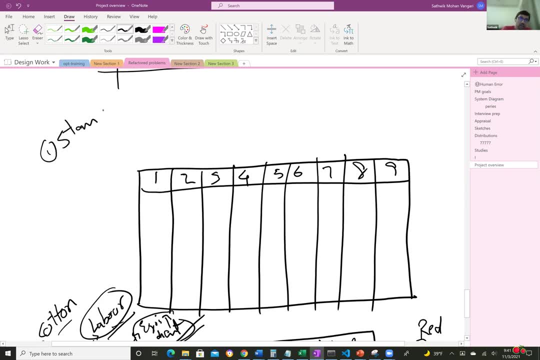 happens with principal component analysis. there are a bunch of steps that principal component analysis does right. so first it standardizes your values because the model is sensitive to variations. then it looks at picking up. you know what do you call it. it looks at decomposing these columns. 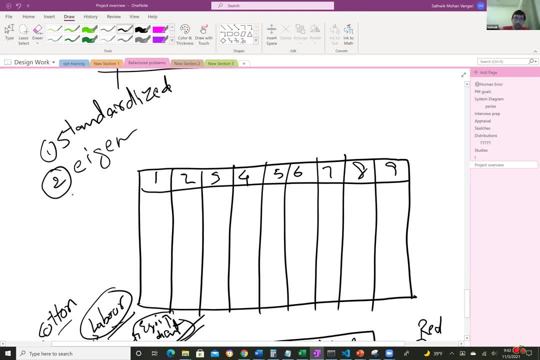 with eigenvectors and eigenvalues, and there are, like you know, a bunch of steps. now let's see how it goes. and then from these decomposed eigenvectors and eigenvalues it comes up with what are called as principal components. then it re-does those particular columns, those 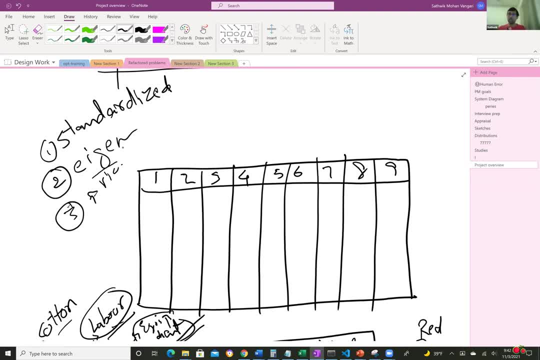 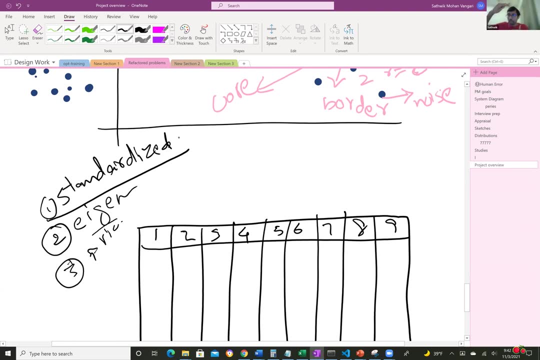 principal components. it repurposes the data so that it's plotted with respect to these principal components. okay, now, what we mean by all of this is. so for a moment, forget about the standardization part. standardization basically means that you condense your values to a range. 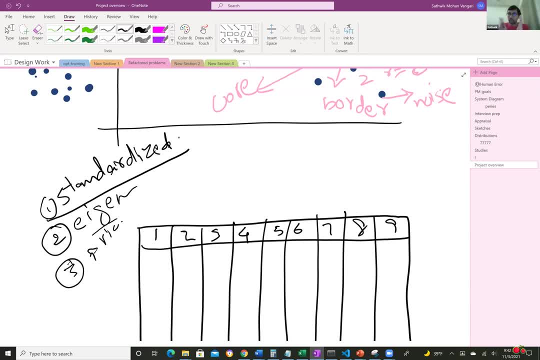 of like minus one to one or zero to one. right you equalize all your values of each column, right you push those values into a zero and one range z score. if you guys remember that right, normalization, standardization, that's exactly what it is. so, um, let's say, first column: right. let's assume that again, this is cost of cotton, right, my and per pound. right cost of cotton per pound the lowest cost of cotton per pound is: the cost of cotton per pound was 0.9. let's assume what was the highest. let's say it was. it went up to 18 dollars. 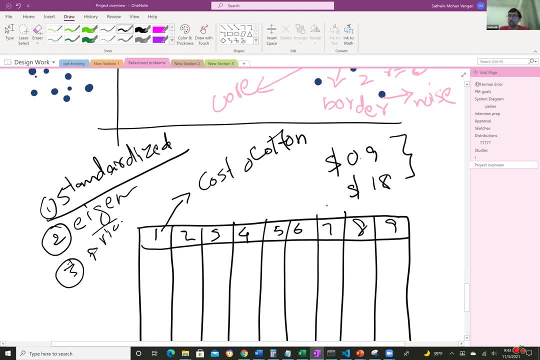 at one point of time. right, let's say, if this is my range, right, and every column will have a specific range of values that it takes. based on the data that you have, you can calculate the minimum value that is there in that column, the maximum value that's there in that column. 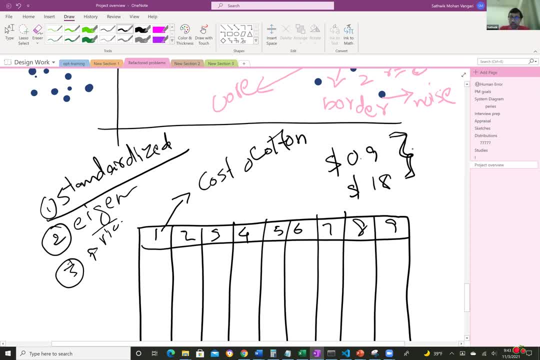 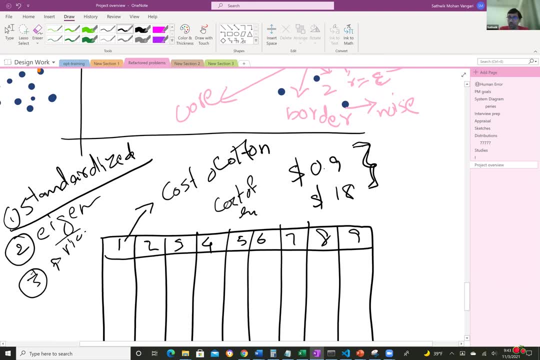 right now, this is a, this is one range. now, cost of labor, let's assume, right, let's say a cost of equipment. let's take cost of equipment, right, cost of equipment might start at ten thousand dollars and might go all the way up to a million. right now, that's a big range. 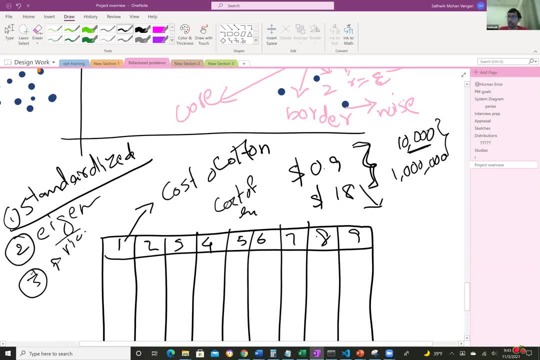 and these numbers are no way comparable to these numbers, right? so this is where standardization comes into picture, comes into play this value. you will condense all of these values and try to represent them between zero to one and the 0.9.. 0.9.. 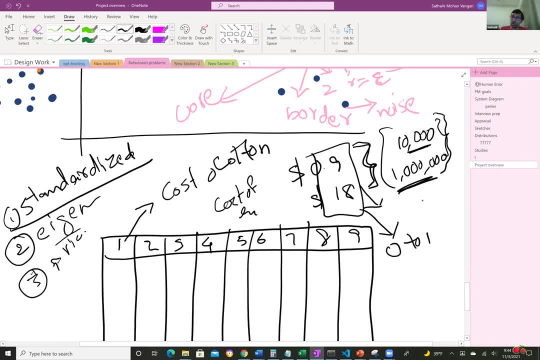 0.9.. 0.9.. is what you will do with this, right, you will condense them and put them between zero to one. that's what is standardization, okay, um, it's just a transformation that you do so that your model applies things better, and it doesn't. it's not thrown off by high variance, right? so for a moment, 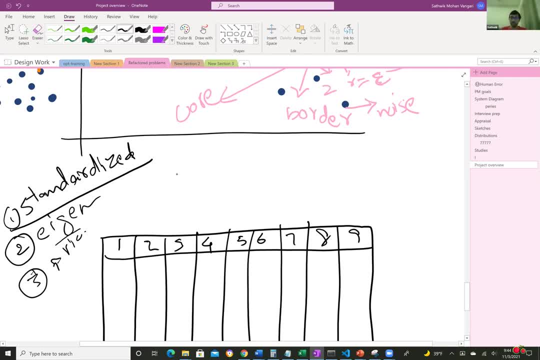 put that aside. that's not uh, that's a processing step. that's not really the core or the core idea of it. now, what are principal components? this is what is important, right? it's a condensation of information, right, in order to generate a new uh, sort of like a new variable that governs your 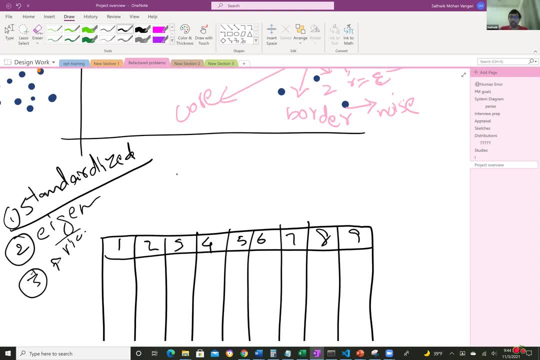 target video, right? so, and what exactly is it? so let's assume that we are trying to, or the model is basically working, we are applying pca and these nine features that we have right, these nine features will be condensed into three principal components: components- okay, so what is each of these principal components? let's assume, assume, 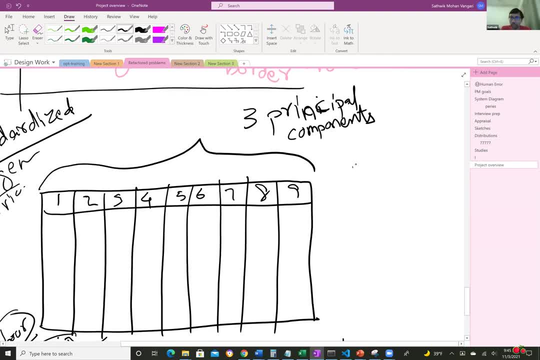 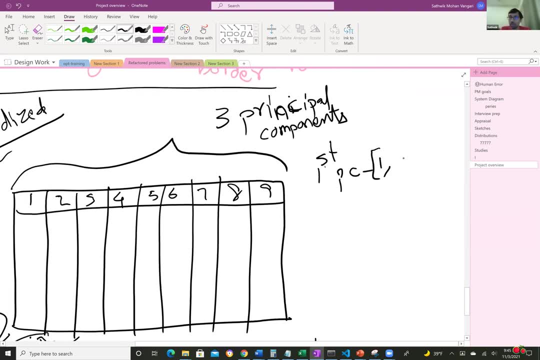 okay, right, that one, two, three here. my first pc or principal component is the set of features, the combination of my first three columns. second pc or second principal component is a combination of four, five, six columns and the third com pc or the principal component is. sorry, i have a question. you say it's a combination of the first three features. 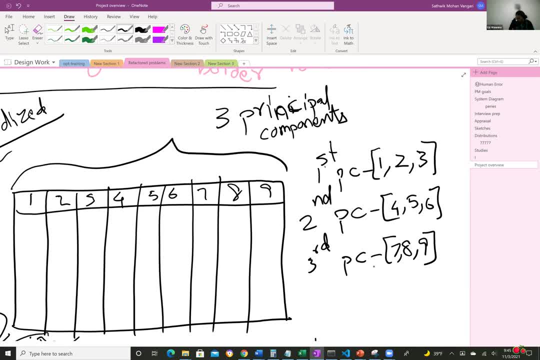 how do we know their features? it's unsupervised learning, you know. how do we know it's right, okay, right. so the better way to remember what we have does it means we have our set of techniques. it is by the self-interview. so that's the answer. 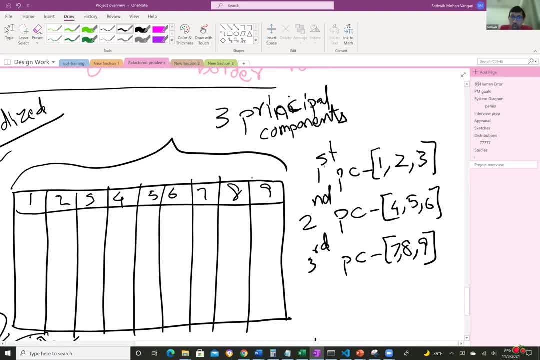 so what does this? tells me: 你先有需要. so now you will download the somebody service tool and get a fairly descended set of four Rhubarb for you, both of your staff and your needs. so, as this you are using for your laptop, is that an independent software, not just your laptop, because i'm not using it, i have my own. 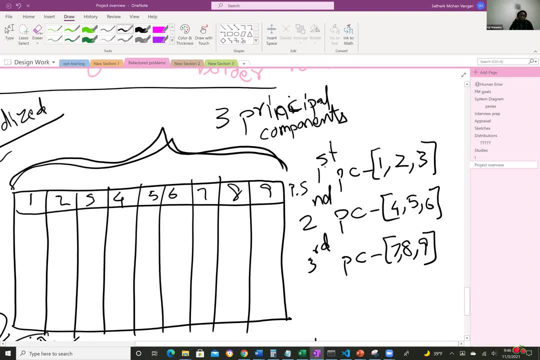 laptop of my own and my books of my own and my checkbooks here, ouch, okay, these are all predictors. you can click on the icon there to check the print contest. right now, the Intel guys is variable. i'm not using my price of shirt here. what am i trying to do? i'm using all the columns. 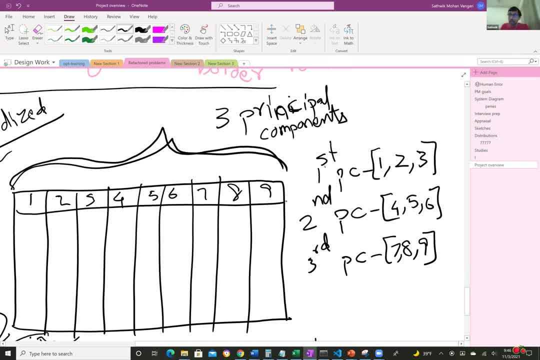 that i'm trying to predict the price of shirt and i'm trying to condense them. okay, gotcha got it right. so if i um okay the others, did you get liz's question? it's a very good question. why am i calling this an unsupervised learning model, while i'm giving you an example of a clear 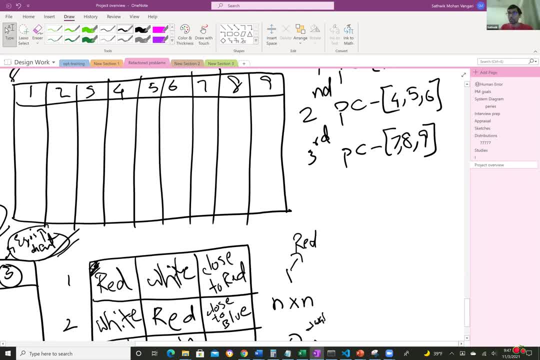 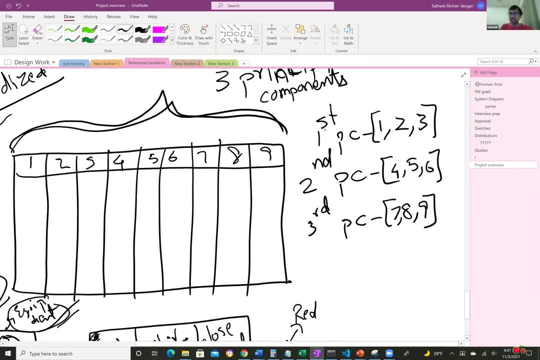 prediction case? right, i'm talking about predicting price of shirt and i'm talking about all these variables, right, these predictors, right. but i'm telling you that pca is an unsupervised technique. how is that possible? right, because while i'm doing pca, i am not considering the 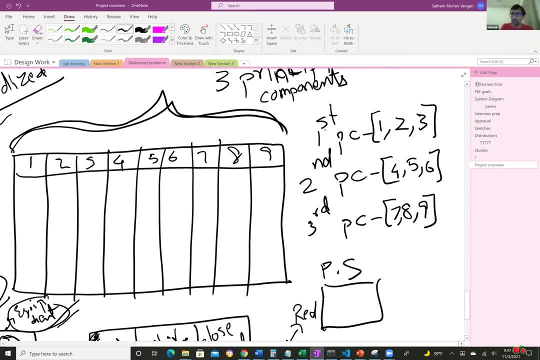 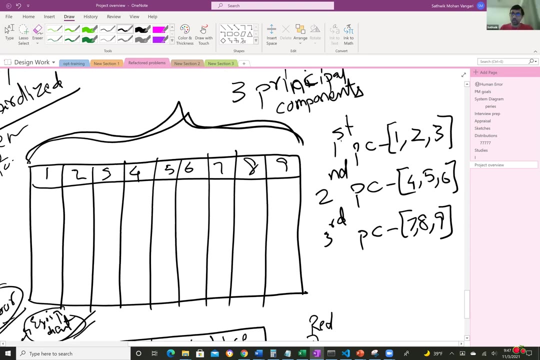 price of shirt. i might have a column with the price of shirt variable right, but i'm not using that yet. what am i trying to do with principal component analysis? i'm trying to shrink my nine different predictors into smaller number of predictors. got the idea, guys, cool. so how does that happen? so pc, a principal component is taking into account. it's, it's. 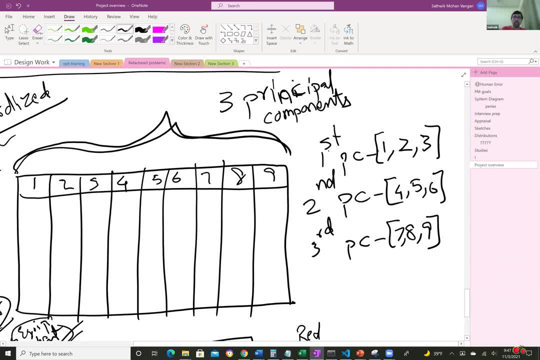 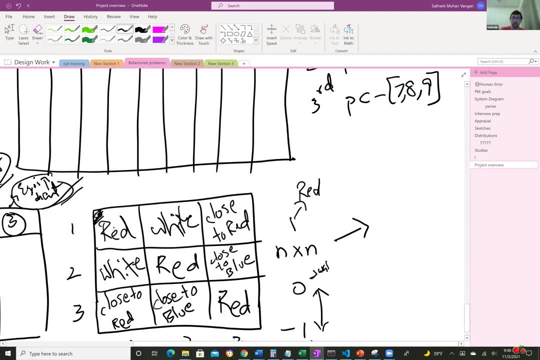 basically trying to condense the information. it's not trying to like. see, when you do this, right, when you do a correlation matrix and you eliminate features, you'll say that, okay, this is important, this is independent, this is independent. i'll keep these two. i'll remove the third. when you remove a feature, you are losing information. 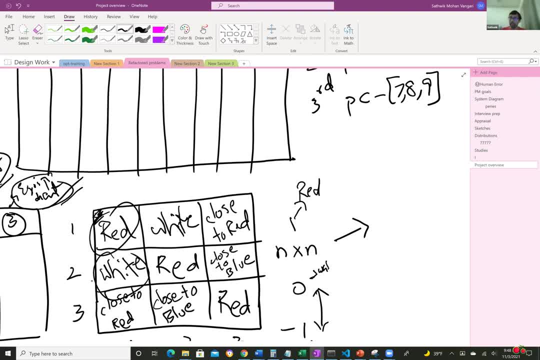 right. you are losing a predictor which has certain influence- or your, on your target variable. and what does that do? when you lose information, it will bring down your model accuracy. you might not have an important component that tells you what your price of shirt could be right? okay, you're getting rid of it. you're getting rid of the information. 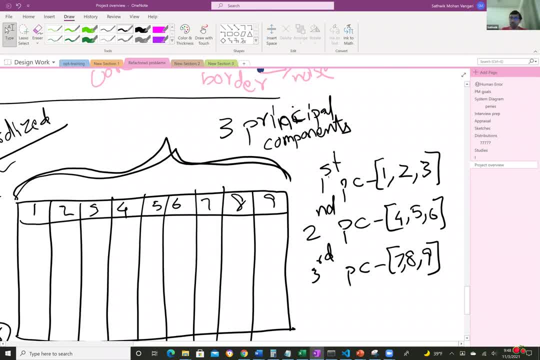 right now, when you have 90 different variables, you're getting rid of the information in a short time and you want to condense them into, like, say, nine variables, only a few of them. it's three variables. when you have three, it's it's. it's it's one level, but when you have 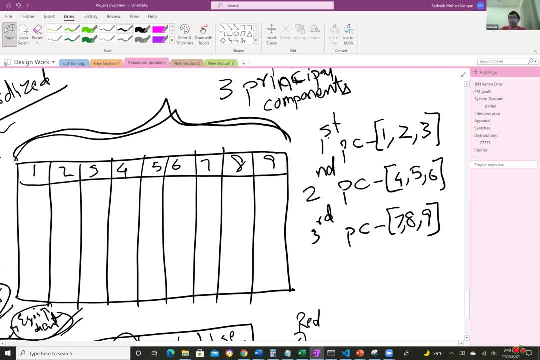 90 different variables and you want to condense them into, like, say, six features. you have to. are you going to throw away 84 features? that's a lot of information to throw away, right? so what principal component analysis does? it doesn't throw away these information, necessarily. 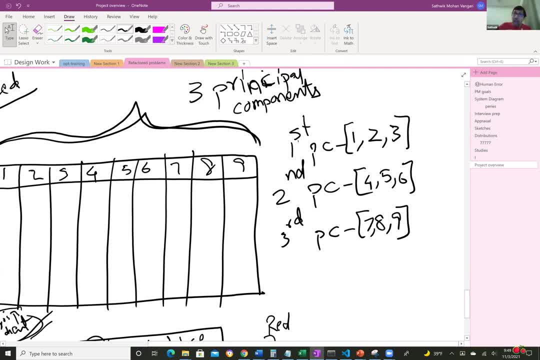 it looks at which of these variables have high variance right. the higher the variance variance it means that the more it might affect the target variable. that's an assumption that PCM makes. So let's say there is one specific column, column 8, where all the values right like over here. 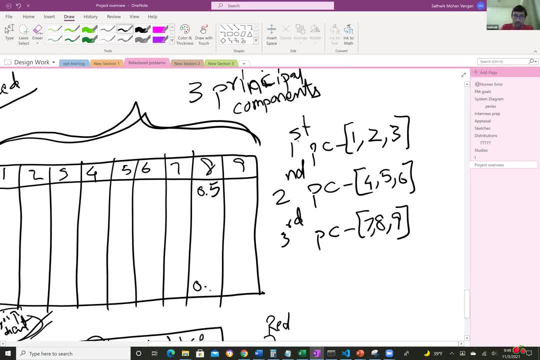 are ranging from 0.5 to 0.6. right, every value is either 0.5 or 0.6, 0.5 or 0.55 or 0.57 or something like that. everything is between 0.5 and 0.6. okay, now, that's not a lot of variation. 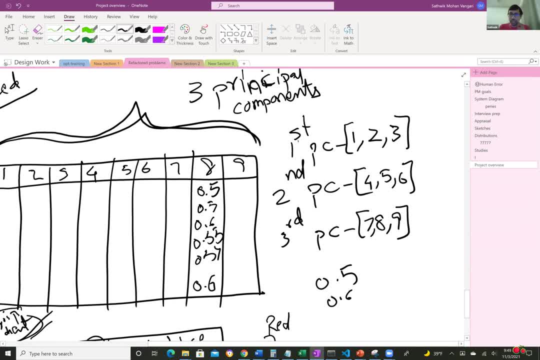 right. there's not a lot of features over there. if you draw a outlier or a box plot, right, you might see a box plot like this right, where all the values are condensed in a very short region. now that means that it might not really have big influence. 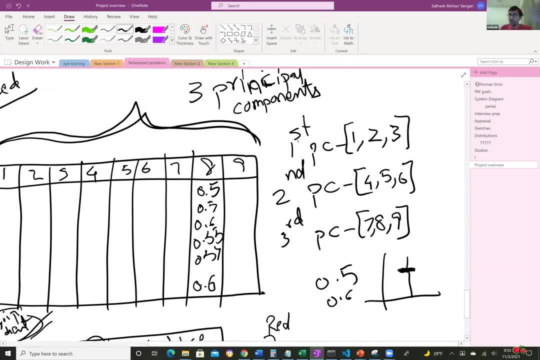 on the price. Now price is changing, but this value is still always between 0.5 and 0.6 right, so no high variance, which means that it doesn't affect the price. it probably doesn't affect the price, so I might kick out 8. I might kick out the column. the model right, the PCM right, right now, assume. 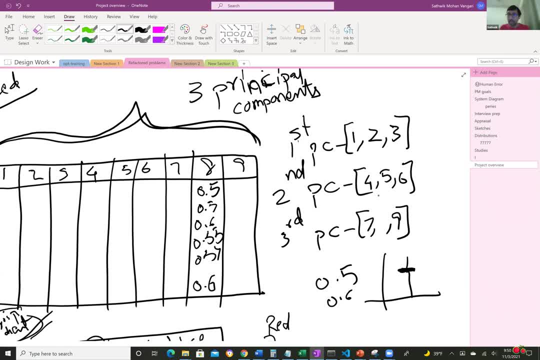 that I am PCA, I am the model PCA and the algorithm PCA. so I'm saying that 8, the column 8, doesn't have too much variation, so it doesn't affect my target, so I might remove it, I don't need it right. and then I take a combination of only 7 and 9, because they still do have. 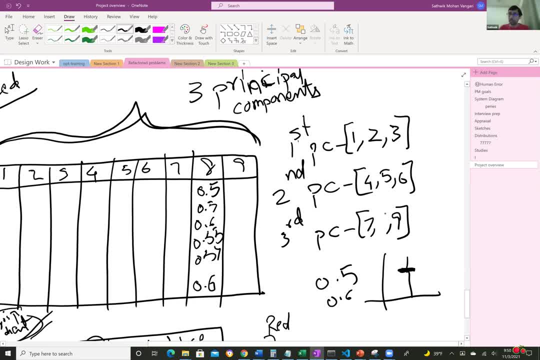 some variation and still they might affect my target variable. right, so that's how it works. so it might take a combination of your features and then it's called a mixture of these features. right, it will take a mixture of these features and then create something called as a principal component, right now, once, let's assume that it creates this particular. 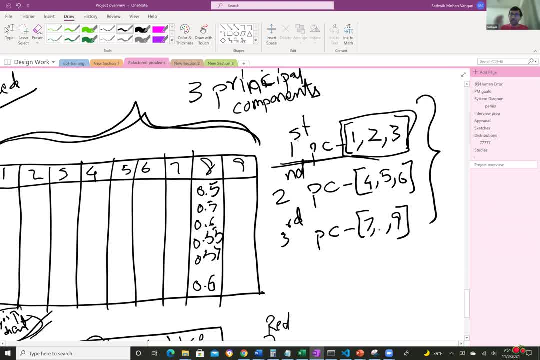 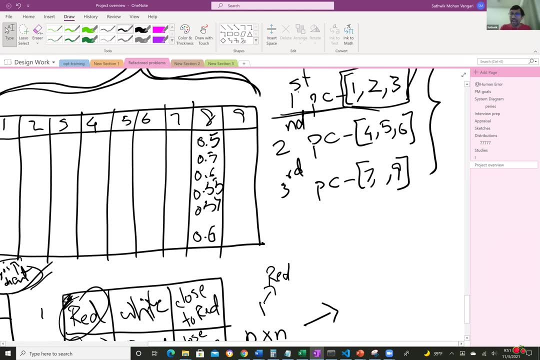 setup. I have principal components. it's eliminating one column, it's taking 1, 2, 3 as one principal component, 4, 5, 6 as another principal component and 7 and 9 as a third principal component. okay, now my multi-dimensional data set right. my 9 data, 9 features or 9 predictors have 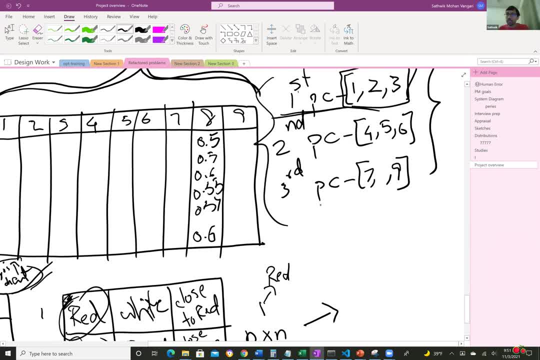 been shrunk to 3 principal components which can be used as predictors. so right, I have 3 principal Components Now. isn't my modest model simpler? Right? yeah, but do you have read columns then? or just or? components are not necessarily columns. yes, so components will be taken in this. they are like columns, but it's not your. 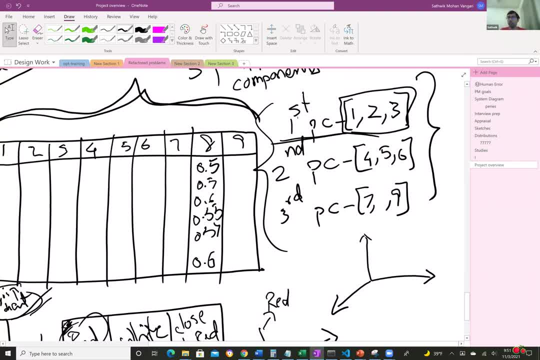 it's not interpretable, right? let's say, for example: what do you, what will you define? is the combination of my 1, 2, 3. columns- right? how do you define that? they don't have a real life definition. it's just a principal component. you call it as a principal component. it's a mixture, it's the effect of these strings. 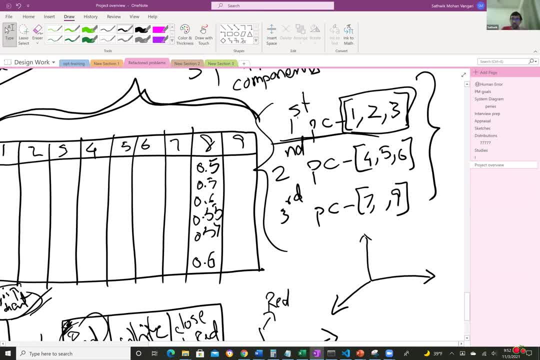 pulled put together. you don't have a real life explanation to it. so you have values. you can visualize it as a column, right, it'll have a bunch of values over there, but you can't explain what those values stand for. making sense, david? yeah, right, so when? when the model generates these three? 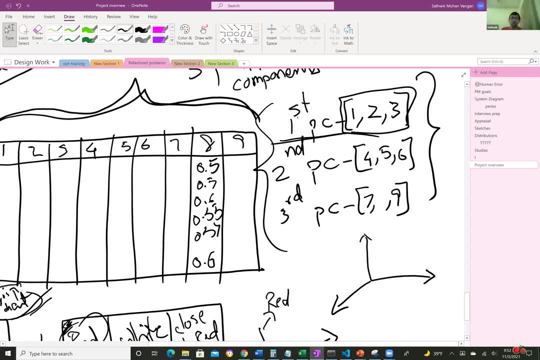 principal components: pc1, pc2, pc3. you can visualize them as columns, but you can't really give them a name. you'll simply say principal component one, principal component two. you don't know how to name them really, right? let's say you took a demographic data data set, right, it might? 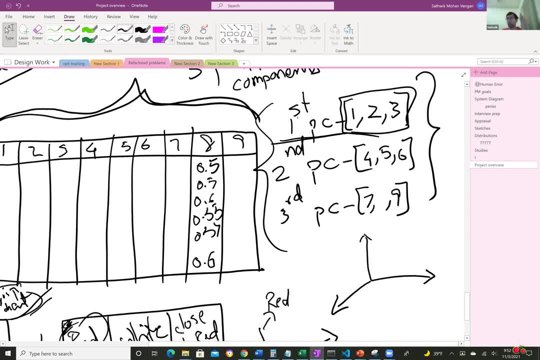 consider age, salary and location as three columns which are, you know, condensed into one principal column, principal component right now: age, salary and location. the combination of this, what do you name it as really right? how do you define this right? so you can't really have a definition to the combination? 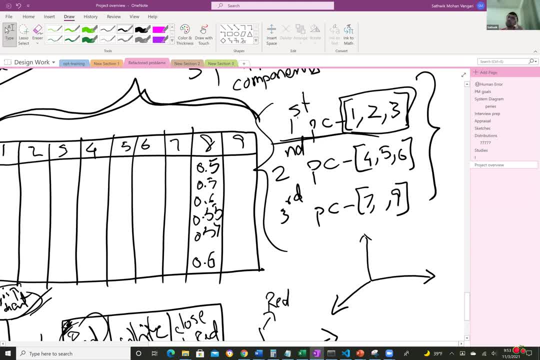 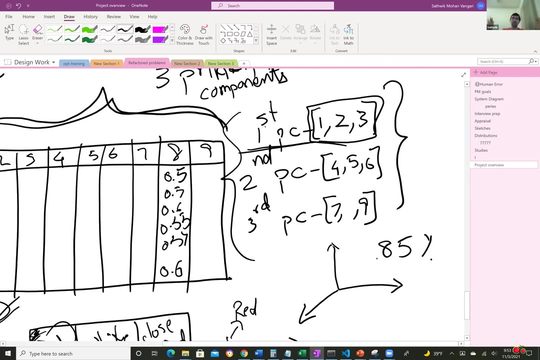 right, it's just called as a principal component. and this is one sort of slight drawback of using something like pc, pca, right, principal component analysis, in the sense that you lose some part of interpretability, which means that now let's assume that i identified, i built the model, and then i got high accuracy, like 85 accuracy, and i'm like happy and i'm like saying 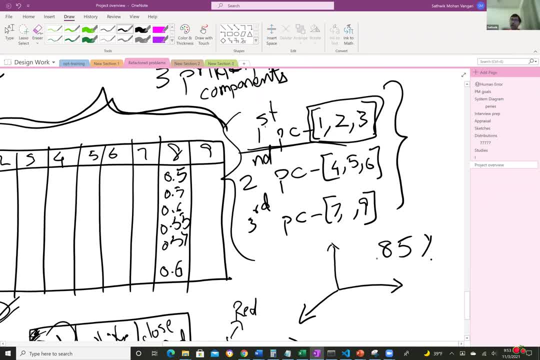 that. hey, with this pca i have three features and i can predict the price of shirt with 85 accuracy. right, but now someone, if my boss, if my manager of you, or if whoever come, has asked me to do the analysis, they come to me and they ask me: can you tell me what are those particular factors that are? 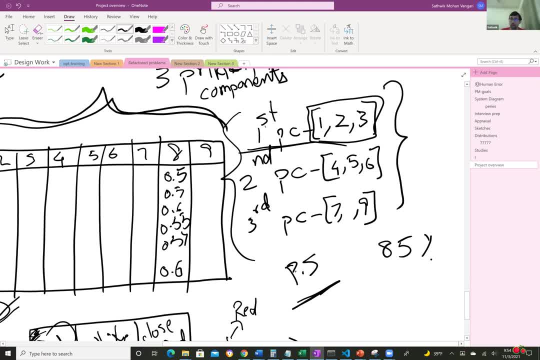 affecting the price of shirt more, right? what are those particular predict factors or predictors which affect the price of my shirt more? i can't tell them right, because all i know is principal component one has a higher effect. let's say: that's what i'm, my model tells me right, pc1 has a higher effect on my shirt, but pc1 is a combination and i don't. 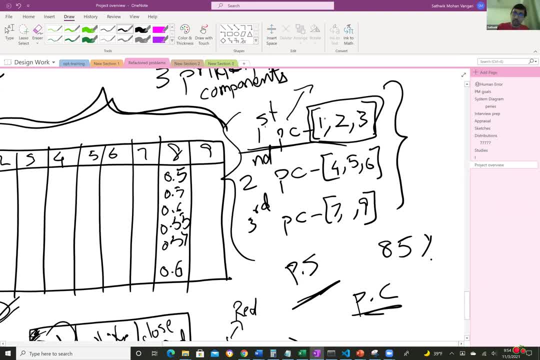 know how that combination is working, was it? uh, in that combination, let's say, there is cost of labor, cost of cotton and cost of equipment. right now i don't know which of these is affecting more. it's a combination that is affecting more. i can tell that, but i don't know which of these. 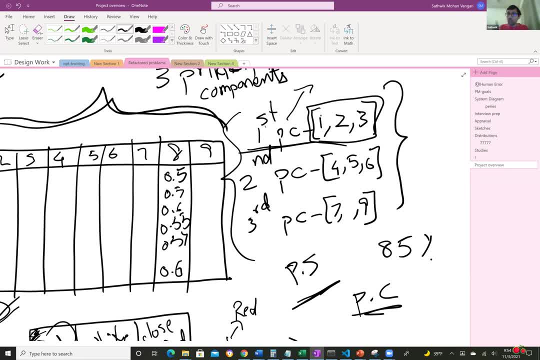 do you guys understanding that right? so you lose a little bit of interpretability when you use a pca, but what you gain is a simpler model, a less complex model, which means that you don't need- uh, you know, you don't have- 90 features. so when you throw all these 90 features to a model like a- 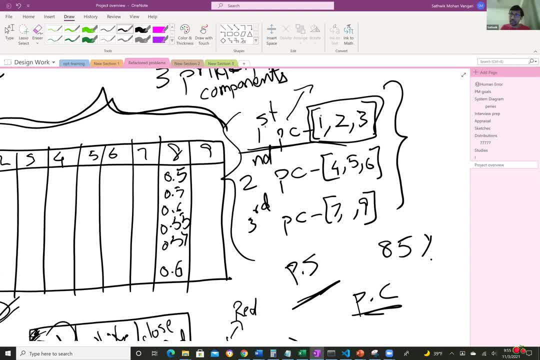 random forest or something. imagine how complex that tree would get right. you had four features in iris data set and you remember how many times it was broken down right. if you have 90 features, imagine how complex a tree it would be be right. so that's why what you do is you first do pca, you condense the data set and then you throw. 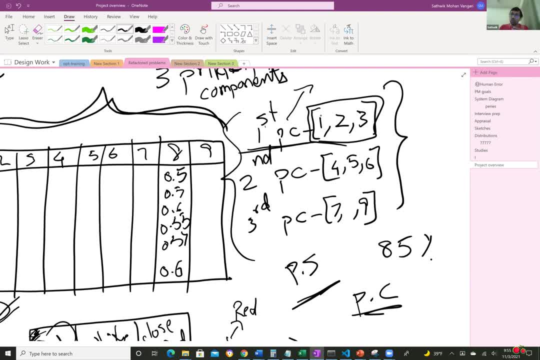 it to the data set, throw it to the model which will use these principal component as components, as predictors, right, and you will get results. you'll get good results, but you can't explain those results, so you are compromising the interpretability. for simplicity, make sense? any questions here, guys? 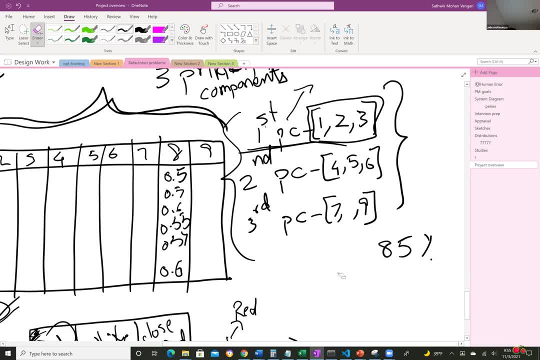 yeah, um, go ahead, jude. so why did you remove the eight? yes, so i removed eight, because all values in this column eight are between 0.5 and 0.6, right, and i don't see too much variation as well. uh, it's not like i'm getting values of. 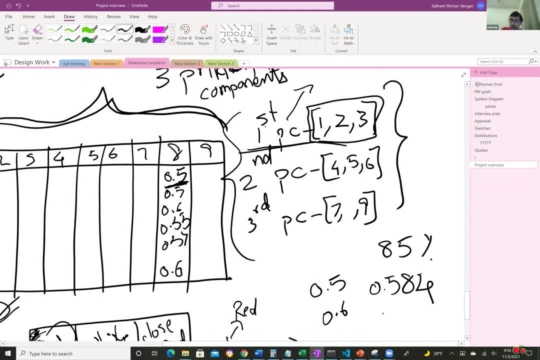 0.864 or something like that. right, all the values are like either 0.5 or 0.51 or 0.52, 0.53 and so on, so there are only really 10 unique values, and every value is repeating in. 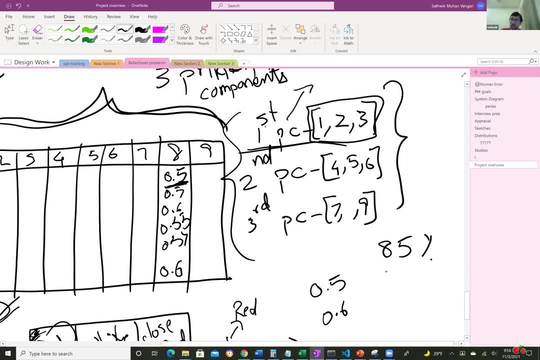 those only 10. those only 10 values is only taking only those 10 values, right? and the variation in my target variable- the price of shirt- is varying widely. this is not varying too much, right? so if i draw a box plot for column 8, right a box plot, the column will look like this: the box plot will look: 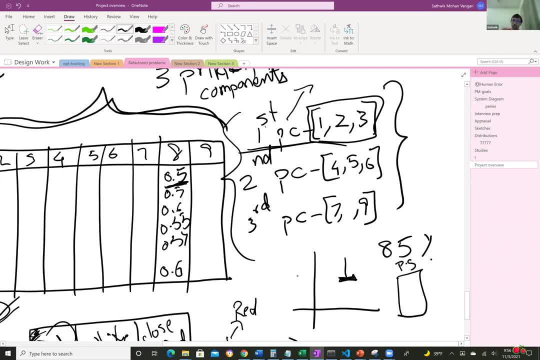 like this, we'll be a very tiny bar, which means there's not Buy Cloth orolt, which means there's not too much variation When I draw a box plot. if my box plot is like this, that means there is a lot of variation. The longer the box, the more the variation. The shorter the box. 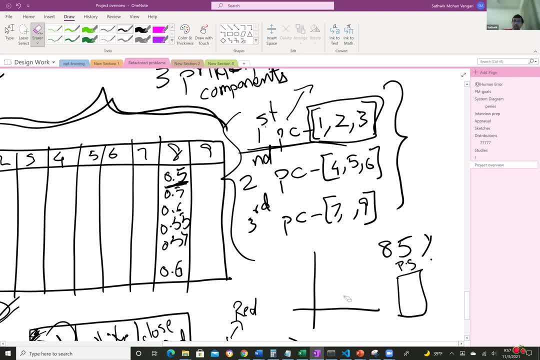 the less the variation or the distribution. So principal component analysis believes that if a column has low variation as compared to the variation in the target column, it assumes that there is high variability in target column. If there is no high variability in target column, you won't be using ML in the first place. Your predictions will be. 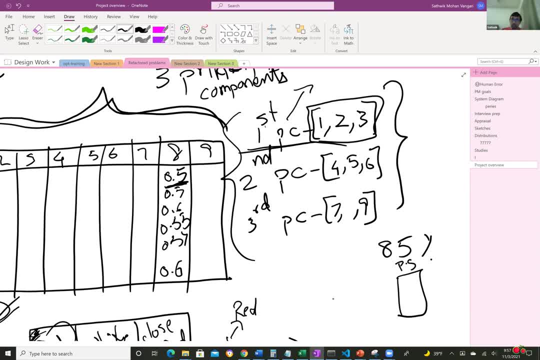 straightforward. So it assumes that columns with low variation can be removed because they won't have a big effect on the end result. That's what it assumes. So in this case, I'm going to draw a box plot. Let me just draw a box plot. Let me just draw. 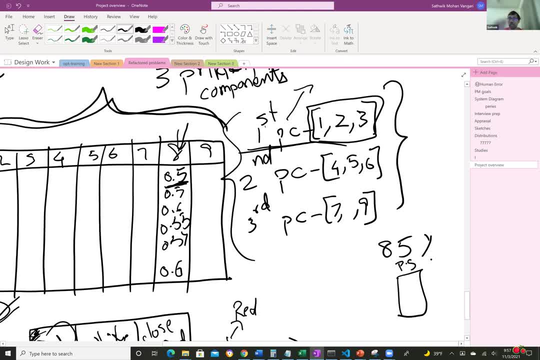 this case, my column eight was an example that I gave to you guys, which has very low variation, And that's why it eliminates column eight. It doesn't even take it into account when it's building its principal components. Jude, did I answer your question? Yeah, Cool. 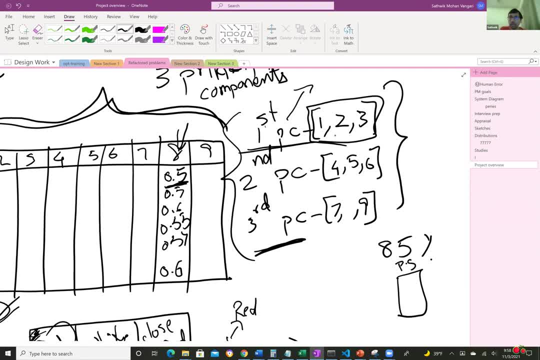 Now also right. So how am I arriving at one, two, three is my principal component, or four, five, six is my principal component, right? This is also even here, right? My PCA model looks at: hey, what are those columns with highest variation? right? So it will take. 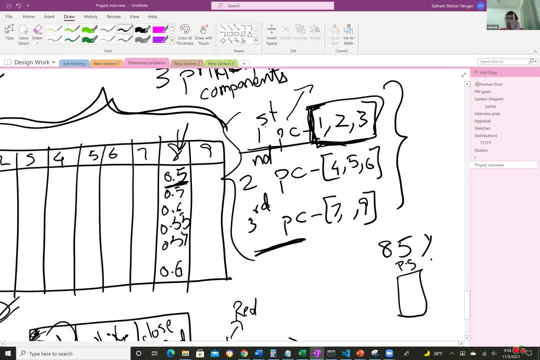 for this case, right, Let's assume column one, two, three have highest variance. It will take the columns with highest variance and build the first component out of that. Then it will take the next couple of columns with like highest variance relatively and then build the second component right, And in doing so 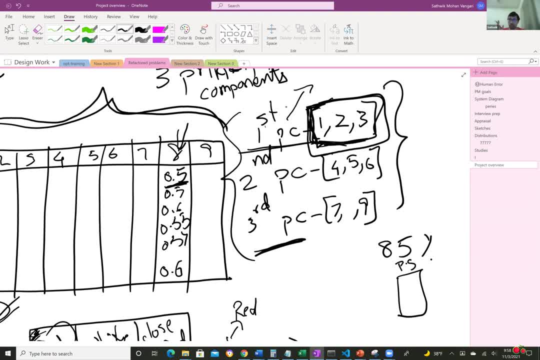 what happens is it will have a certain threshold for variance. How much variance should my column have And all columns which don't have variance beyond that? it will just remove all those columns right, And it will consider the remaining columns which have like high variance, which 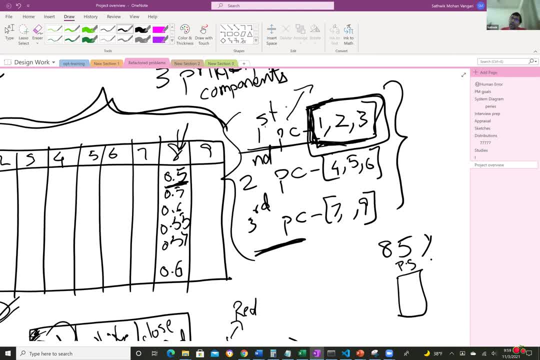 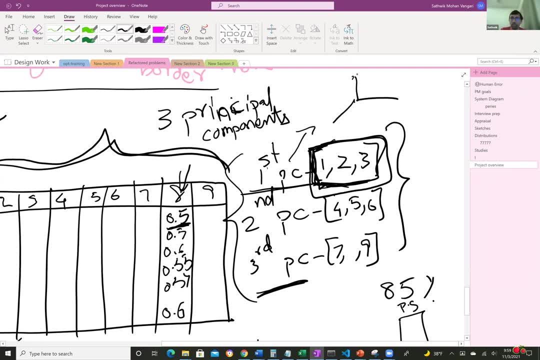 means high effect or high influence on my target- and combine them to build what are called as principal components. And then what it does is it finally builds the data set in a three-dimensional axis, or two-dimensional axis, depending upon these. each axis is principal component, right? This is where it plots my final data set with the. 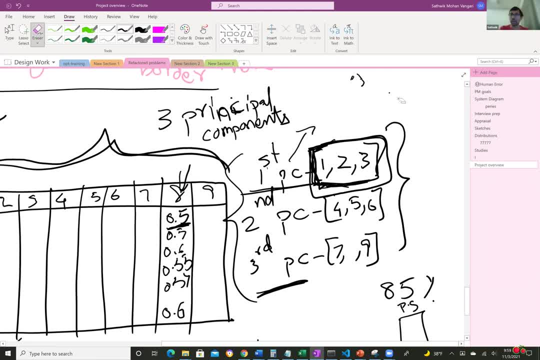 principal component, And then that's how it uses and predicts your data. Okay, Now how does it arrive at these components, How does it arrive at these combinations? That is where eigenvectors and eigenvalues come into picture. It's that's why we included it in the curriculum in DS2, right? So in DS2, we covered the topic of 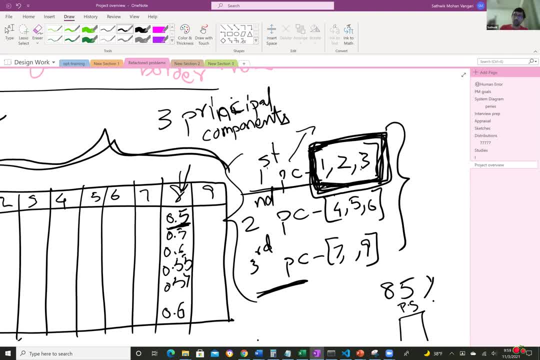 eigenvalues and eigenvectors and that's why we did that right, So that eigen decomposition is what basically happens. That's the process. You don't need to know how it works and all of that- I mean the details of like how eigenvectors and eigenvalues are calculated- you guys can refer to. 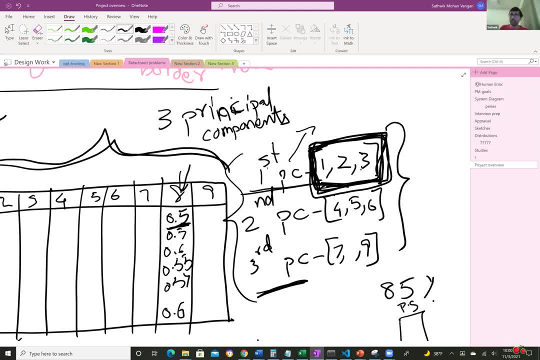 it right And that kind of tells you, like, how this works. but this is basically how it works right. It takes in combinations of columns. It leaves out columns with lower variation, picks columns with high variation. The combination of these columns are called as principal components, and that's how it's reducing the high dimensional. 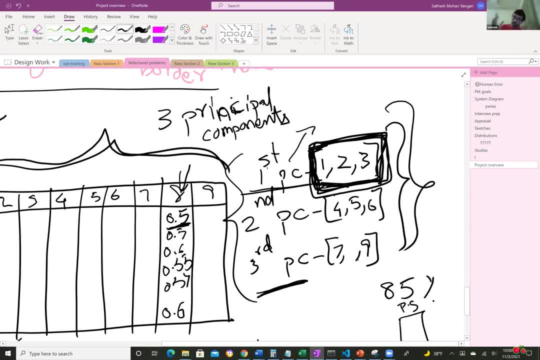 data into lower dimensions, Then repurposes your data in terms of you know, repurposes your data in terms of these principal components, And that's what you end up with, That's what you use in your end result, in your supervised model. But the unsupervised technique- 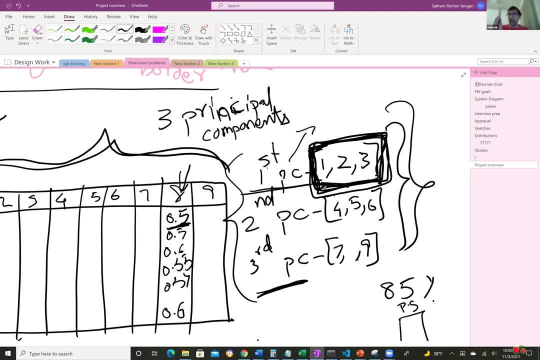 the principal component analysis itself condenses, say, 9 or 18 or 90 columns into 5 or 6,. right, That's where the model stops: Principal components analysis model. the job of that is to construct these principal components, each of which is a combination of columns or combination or condensed information. right. 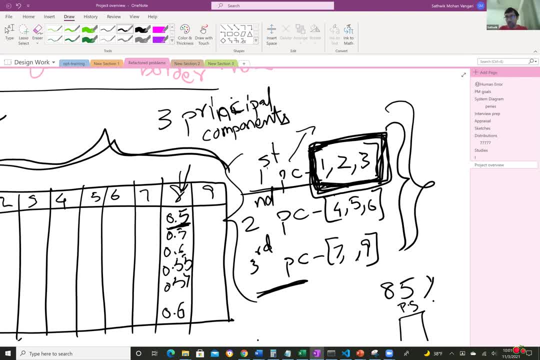 And when it gives you these principal components, its job is done. That is why it is unsupervised model. It doesn't have to deal with the target, So it's not looking at labels, It's just looking at your predictor set. I posted a link on chat before today's class even started. Actually, I was. 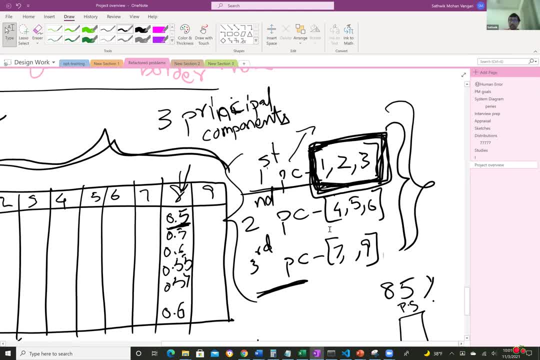 trying to look at the article which had like one of the most simplest explanations and the best explanations of PCA. So I stumbled at one article which I felt was like. so he writes in that article right up front, saying that I am not going to talk about the math of this. 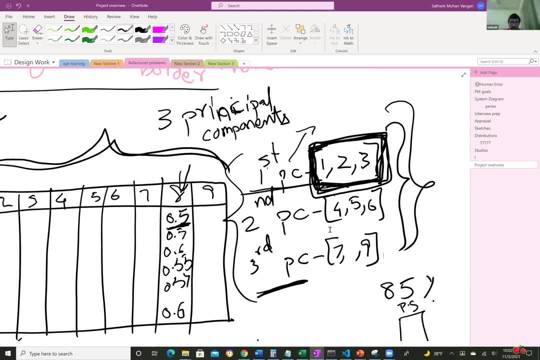 of how PCA works. So he doesn't talk about eigenvalue decomposition. He doesn't talk about what eigenvalues are, how it's calculated and stuff. In simple, plain English he tries to explain what exactly PCA is and how it works. So I found that article is one of the best. 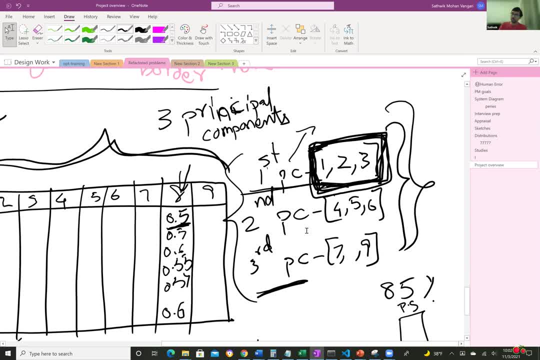 explanations in a simpler fashion. There are a lot of PCA articles I've read, but they don't have an explanation that simple right, Because all of them go into the math of things. It's very difficult to follow those kinds of things with the amount of math that is required. 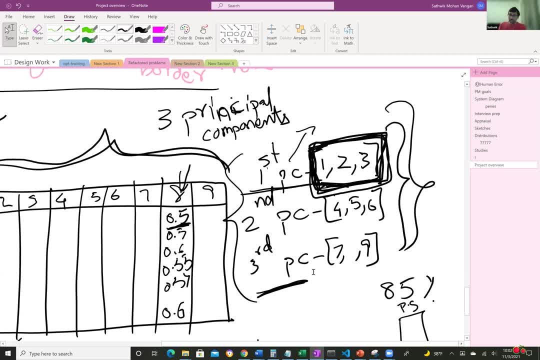 right, But read that article. I'm pretty sure you guys will grasp some concepts, some of these concepts. In the next class, as we do, we will do a revision of PCA. but read up your PCA notebook, read up the article that I posted. 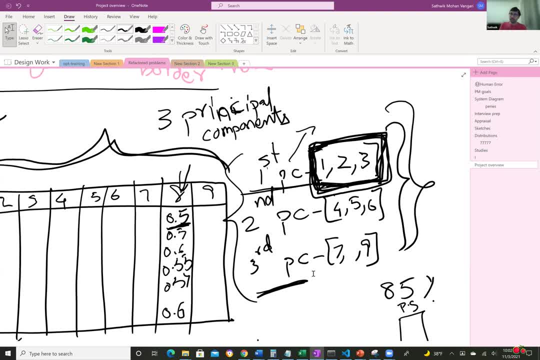 and try to understand PCA again. We'll talk about PCA again in the next class. Okay, Sounds good. Yup, Fuses blowed. Good night everybody. Fuses blowed Question. Yes, You don't have a question, Jude. 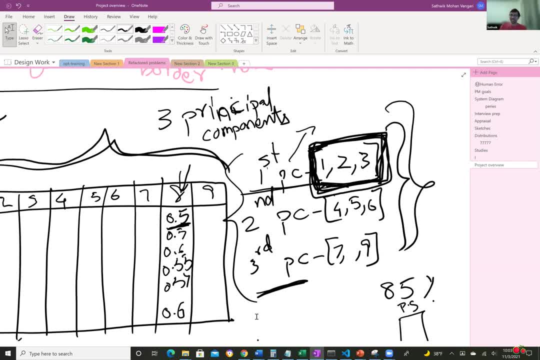 Go ahead, Jude. If you do have a question, go ahead. I don't have a question. You don't have a question. Or are you afraid of Liz? I don't know. He just wants to upset me. Cool, That's the reason why I'm also stopping the class here. 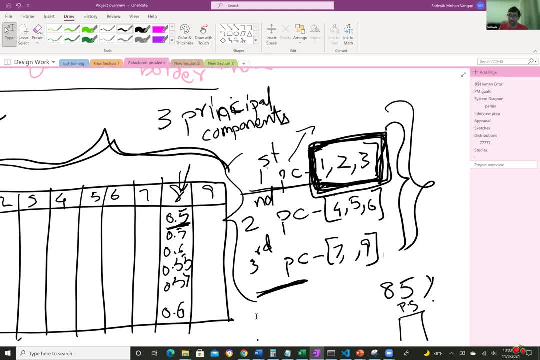 I know it's probably a little too much to grasp, but trust me, It gets better. Read the article, Read your notes, Try to attempt the lab. Come back in the next class. We'll revise this concept once again. Try to. 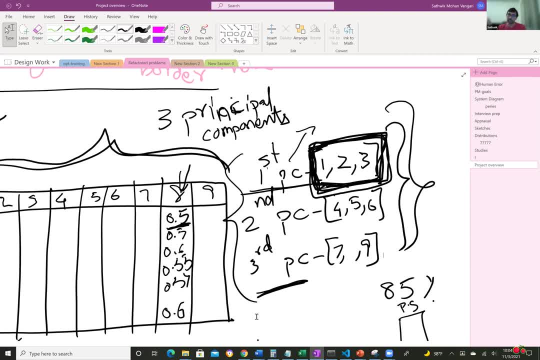 When you read this, try to remember the class. Try to remember what we talked in the class. It'll all make sense. It's just a combination. It's a combination of multiple columns. You're just trying to reduce it. You're just trying to reduce 90 columns to 6..